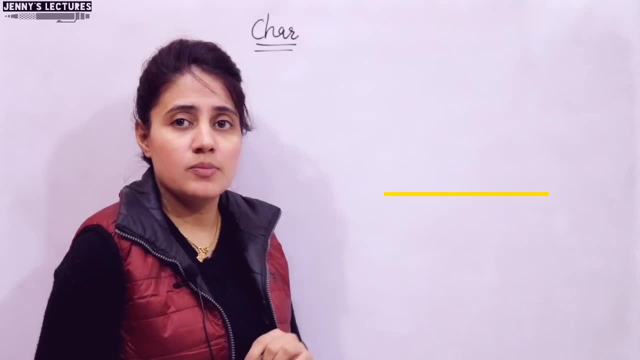 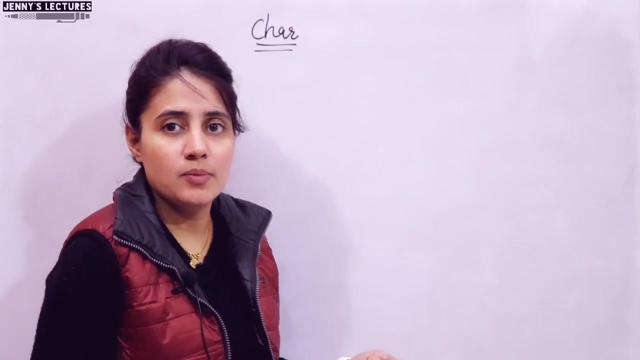 you can say with programs. In this video I am going to discuss about character datatype, all about a character datatype. the memory is taken by character datatype- signed character datatype, unsigned character- and with a program we will discuss like how a character would be stored in computer memory, because computer can only understand what The language. 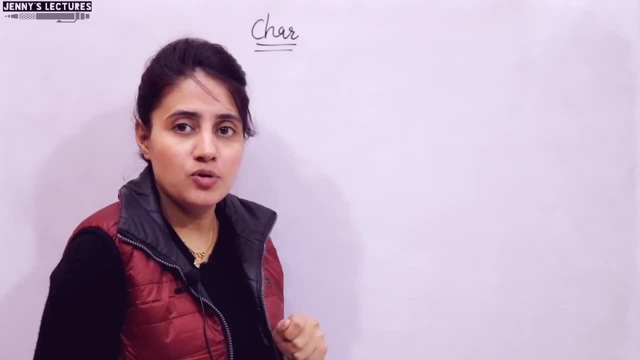 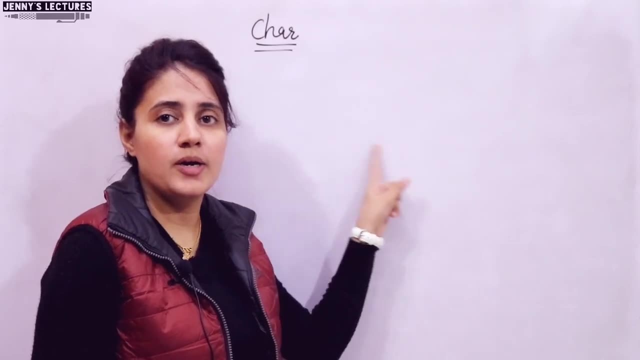 of zeros and ones, so how the characters are to be stored in computer. that also we are going to discuss. what is that character system? we are going to discuss With a program. I am going to discuss, like when you will print anything, any character, then what should? 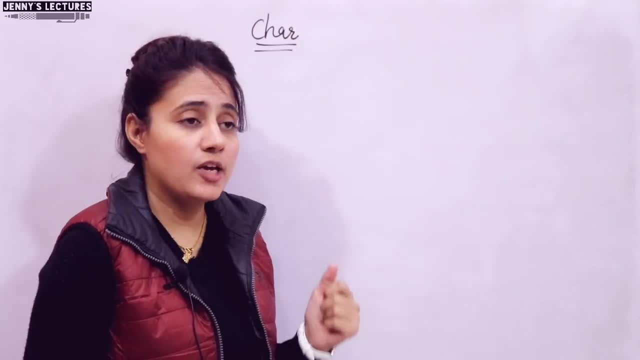 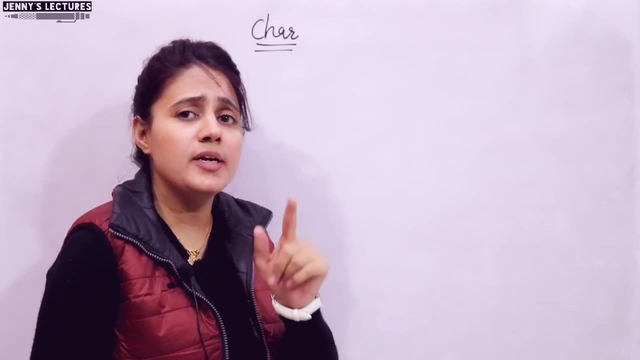 be the output when you will use different format specifier. like if you are printing with %d, then what would be the output? if you are printing with %c, what would be the output For a character to print? a character format specifier is what %c, %d is for integer. 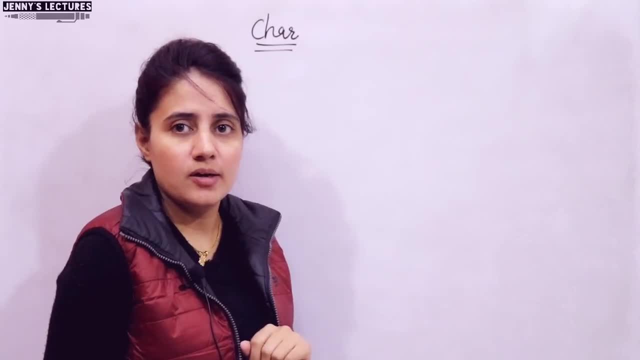 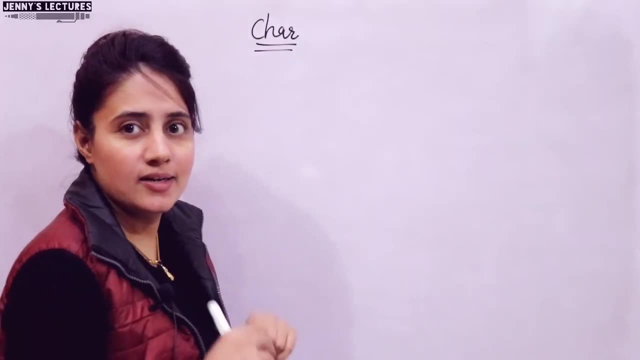 signed integer. %u is for unsigned integer right. everything we are going to discuss in this video, right? So now let us discuss about this char datatype character. char means character we represent with char. this is what keyword in c: to represent a character. 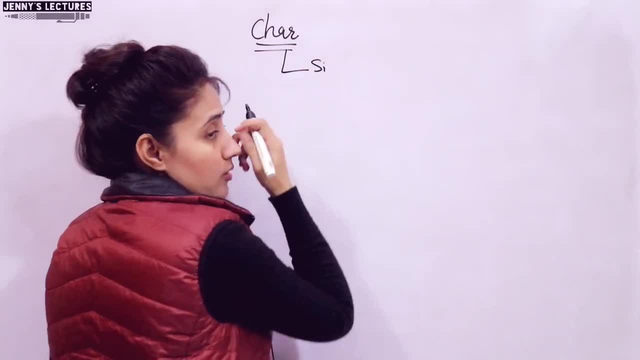 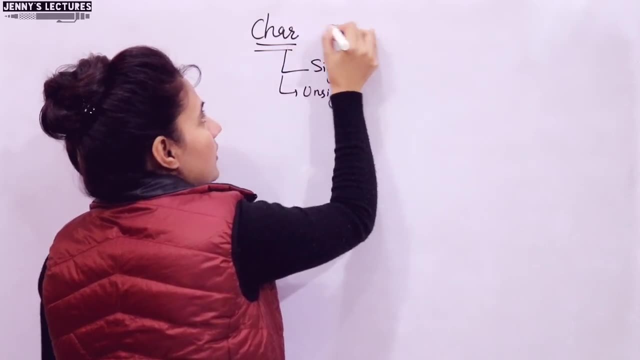 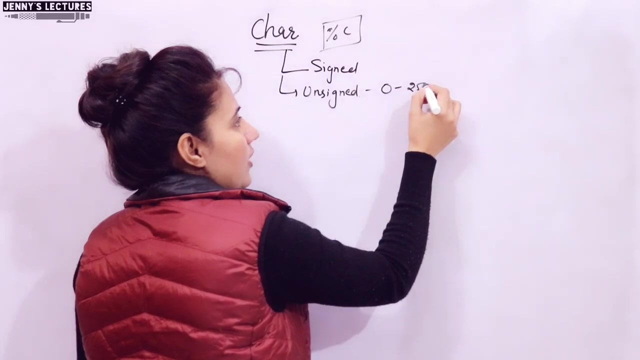 datatype And this is of. we have modifier here that is signed and unsigned, And the format specifier for character is to print a char. the format specifier is %c. Now what is the range? range for unsigned is 0 to 255 and for this it is. 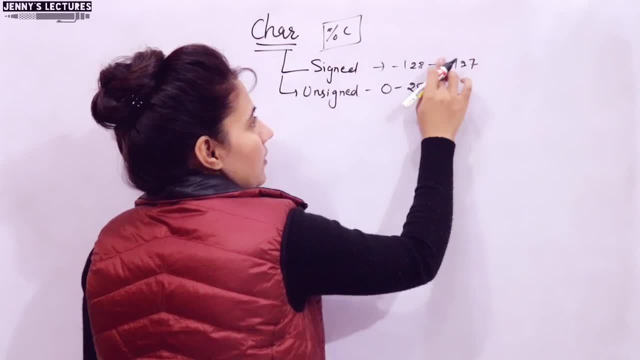 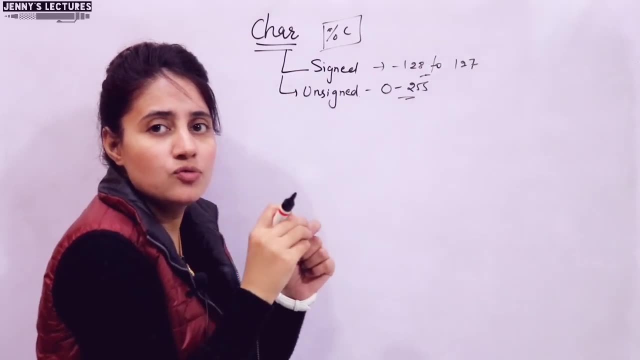 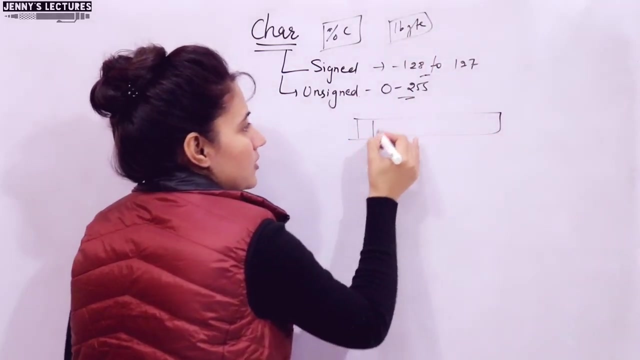 minus 128 to 127.. Why this range is between this see for a character, the memory value which is required. the memory which is required is what? 1 byte, only right. 1 byte means 8 bits. now 8 bits. I am going to represent like this: the minimum value you can store here is what: 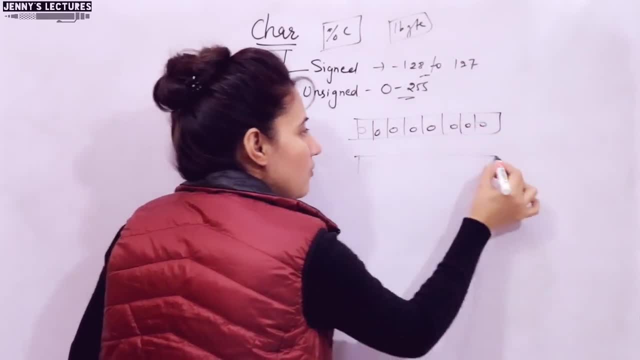 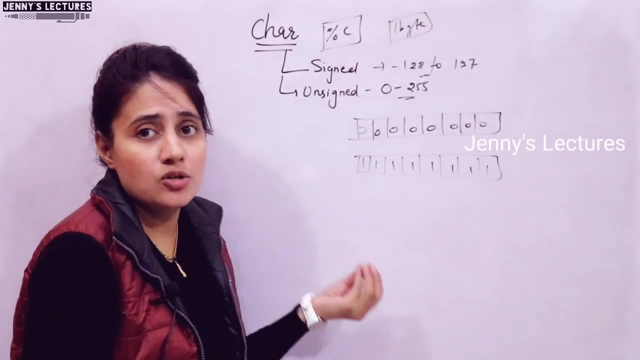 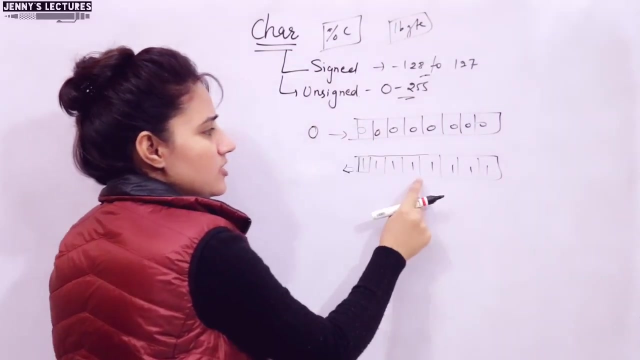 you will put 0 in every cell and maximum value you can store here is what 1 you can store here, because only 0s or 1 we can store. so, according to this, this value is in decimal. if you convert it, that would be 0 and, corresponding to this, this is binary number. 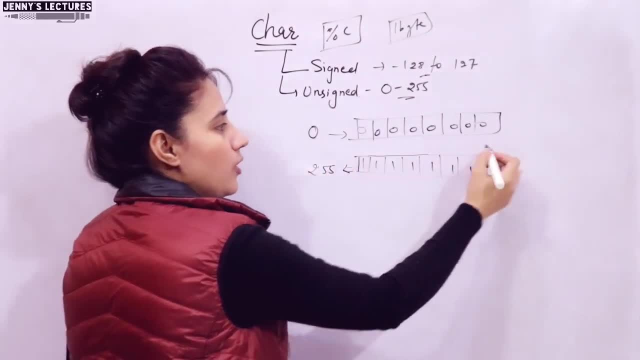 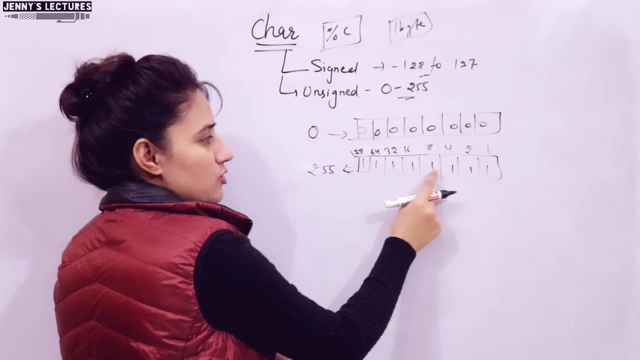 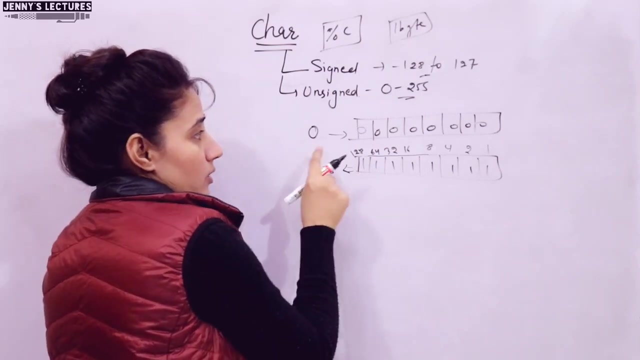 corresponding to this decimal number is 255, have to convert it. this is part of number system actually, so every at every place we have one. so just add these numbers and you will get a sum of 255. that we will discuss maybe number system in some other video. now, minimum number is 0 and 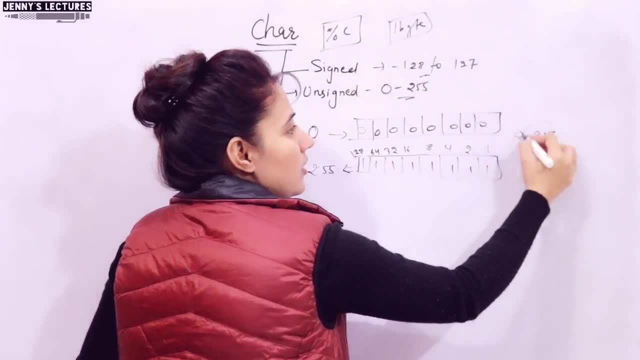 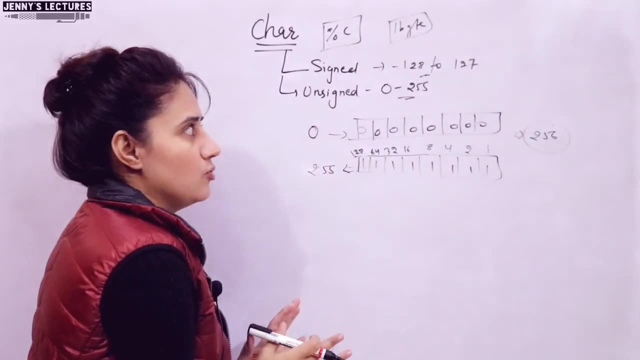 maximum is 255. so total number you can store here is 256 characters or numbers. you can say now this is for unsigned, because here we are having only positive values. now when you convert it to a decimal number, you can store here is 256 characters or numbers you 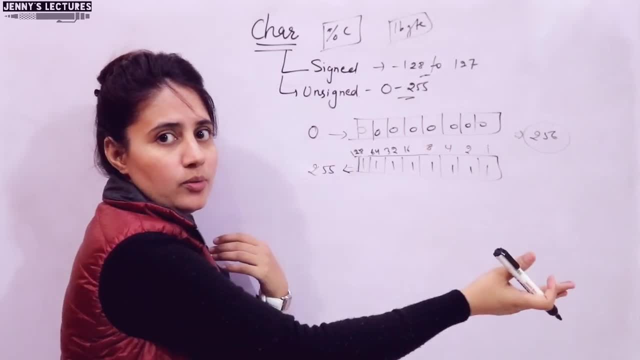 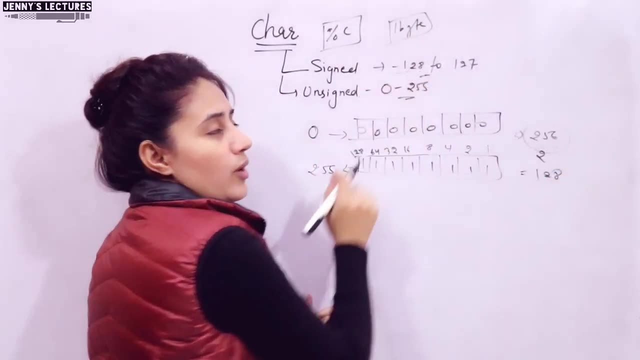 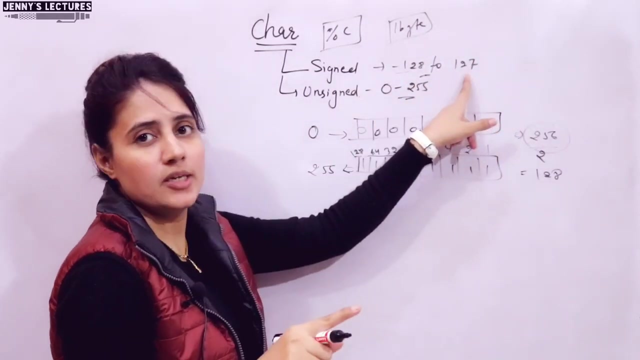 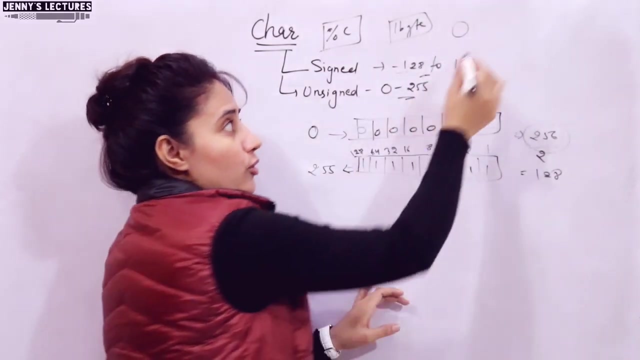 can come to sign, then half value would be of negative side, half value of positive side. so if you divide by 2, then it would be 128. so here you can say: from minus 128 to minus 1, then 0 to 127. that is why here 127. why so? because in positive side we are also including 0. we are not going to 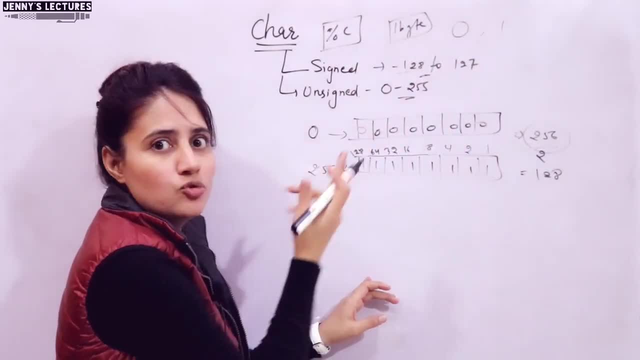 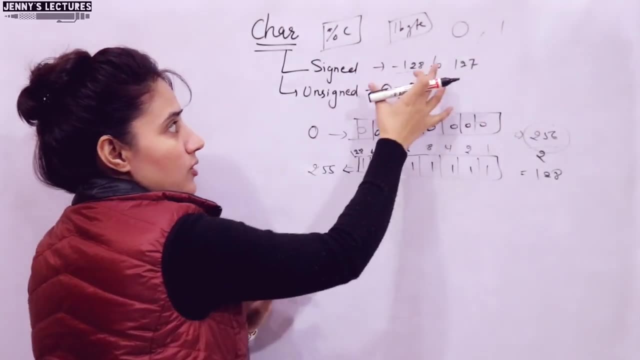 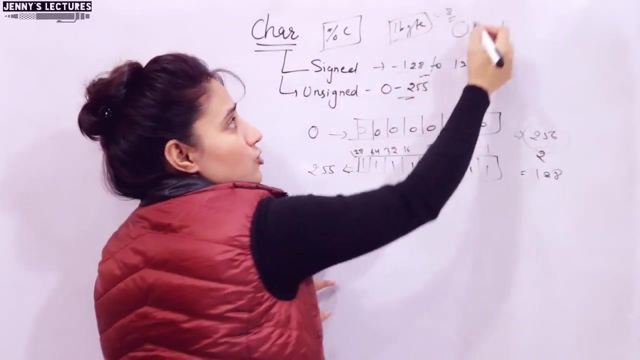 start from 1 only because in negative side we are going to start from minus 1. that is why the range is for minus 128 to 127. only here is no, it is not 128. I hope you got the range. why the range is between this and you can say from this also: if it is having 8 bits, then how many numbers it can store. 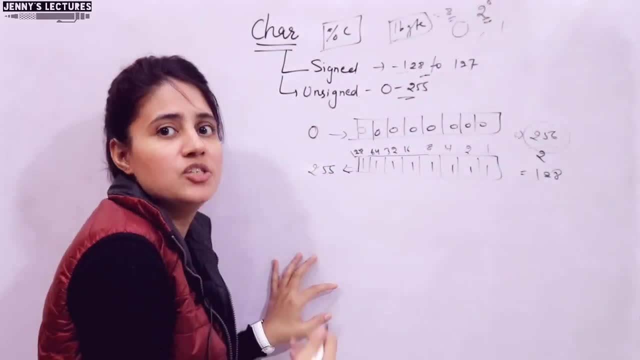 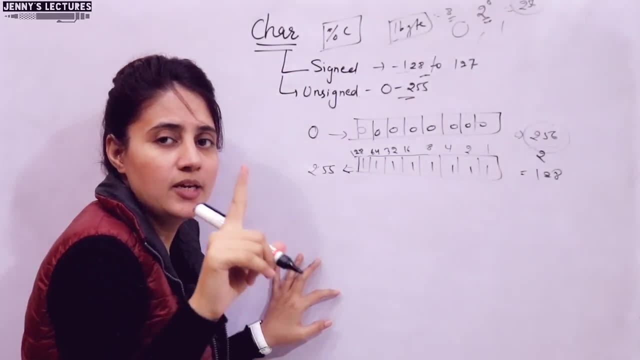 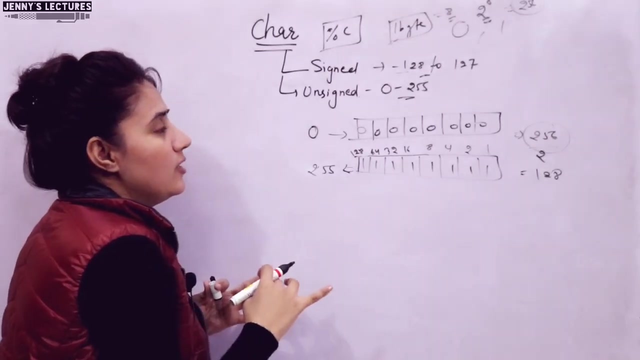 2 raised to power 8, how many combinations can be there? and 2 raised to power 8 means 256 values we can store right with one byte memory in one byte memory right now. let's come to that how the program we write would be converted into that zeros and one form, suppose I am writing here. 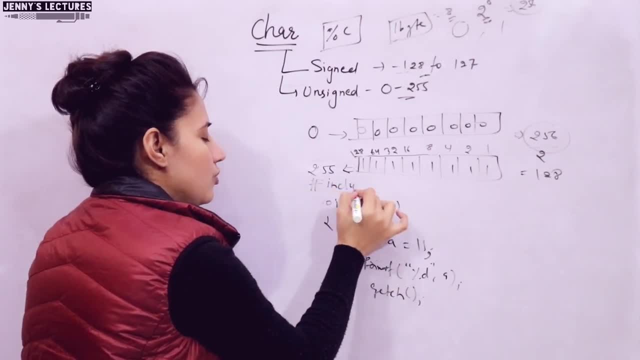 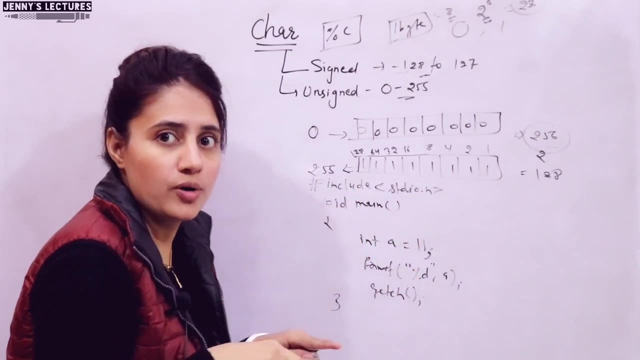 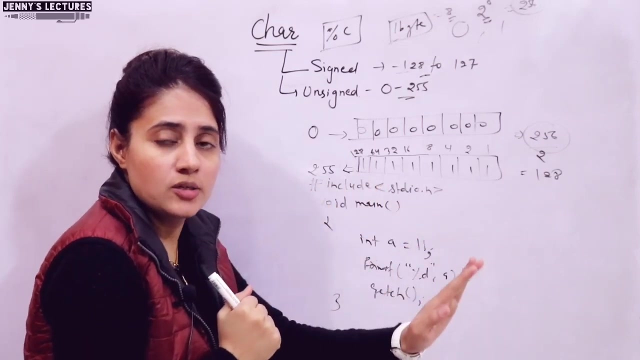 now. now this program- and these are header file hash, include stdio dot H. and forget says you have to include hash, include conio dot H also. I am NOT writing here that file now. this program would be converted into first of all binary zeros and ones, then it can be stored in computer memory. we cannot 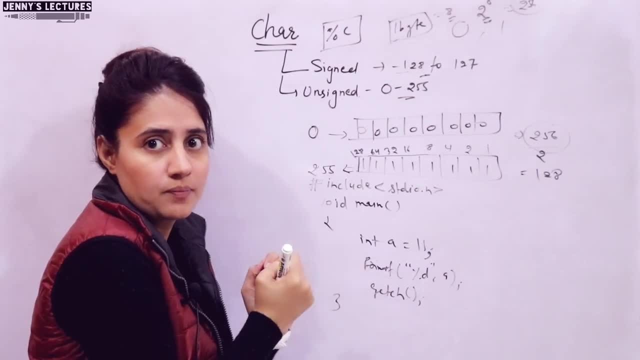 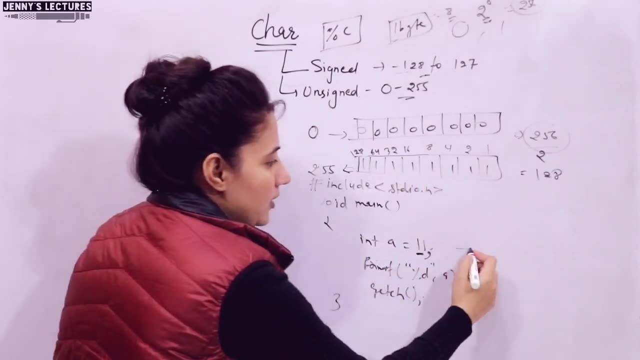 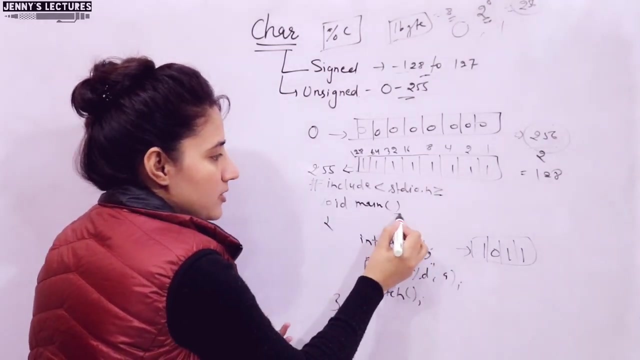 directly store this program into computer memory. computer is not able to understand this thing, right. so now, ok, 11 can be converted into decimal by this number system. 11 we can represent 1, 0, 1, 1, but have you will represent this, this symbol, have you will represent this symbol into memory in zeros and. 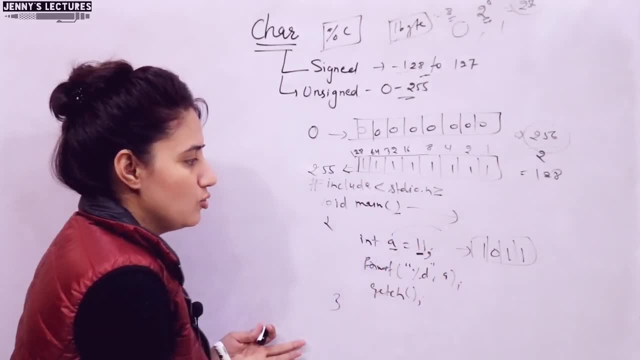 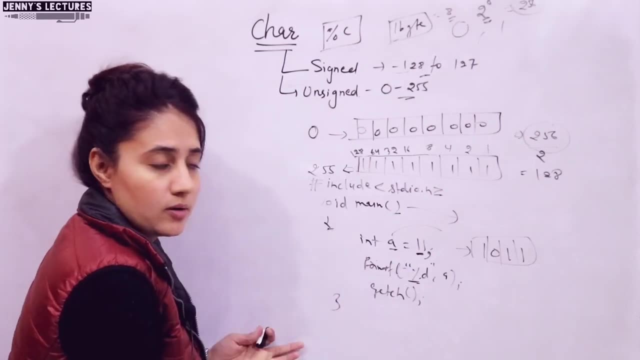 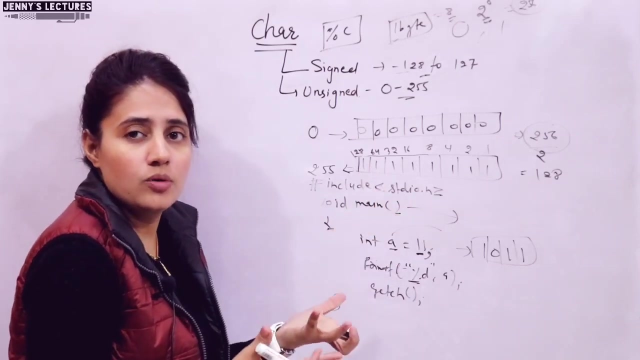 one forms have, you will represent this a in zeros and ones forms have you will represent this percentage quotation mark, this symbol, this symbol, this is number system is just for numbers. how you will represent these characters, these special symbols into the computer memory. for that we use what character system for this? 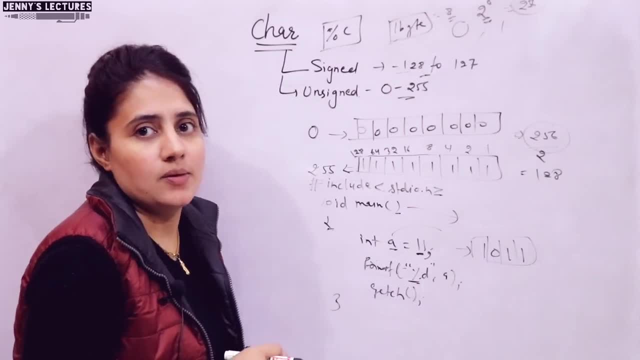 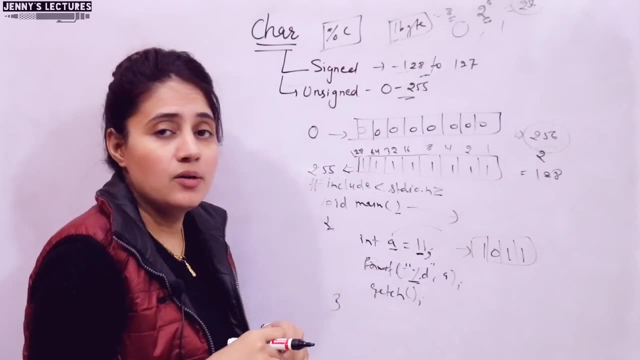 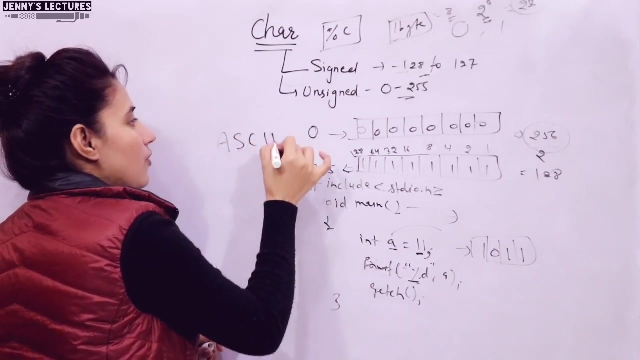 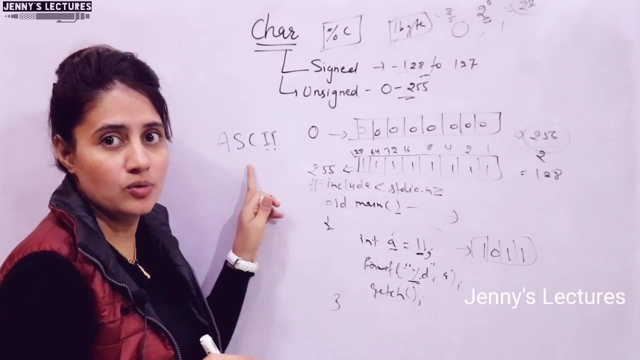 number system is there for that, we will use character system. now many character systems are there: bcd, ebcd, ic. ibm is having its own character system and the way the very popular character system is what? sky character system, american standard code for information interchange, that is a sky character system. this is of two types: seven bits also, eight bits also. 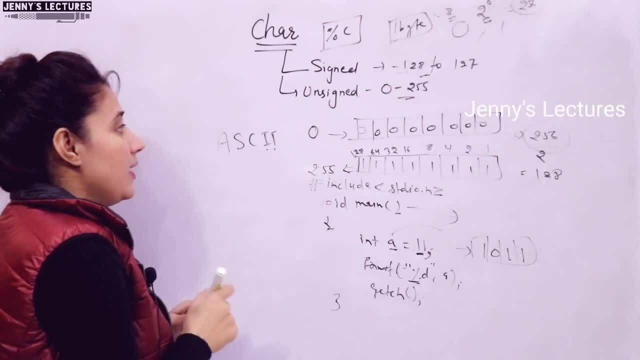 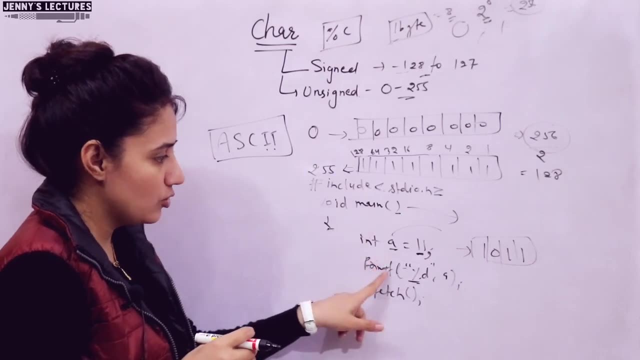 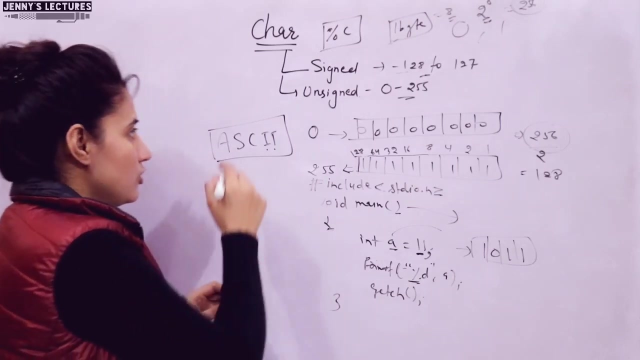 maybe all character system, we can discuss in some other video, but this is a sky character system, is what it is used to represent. this text, this is what text, or you can say the character, into computer or any telecommunication machine, these type of devices this was developed for, especially for. 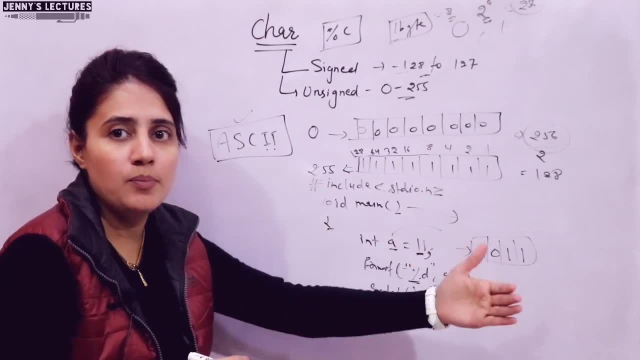 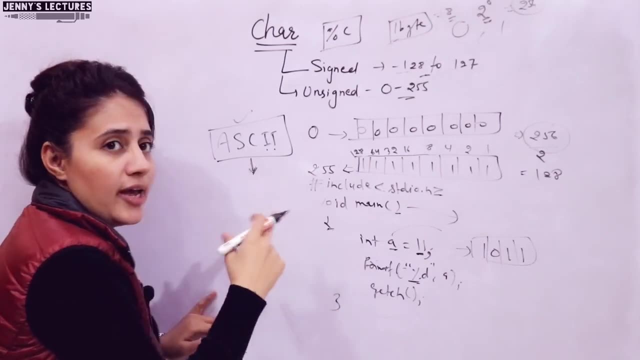 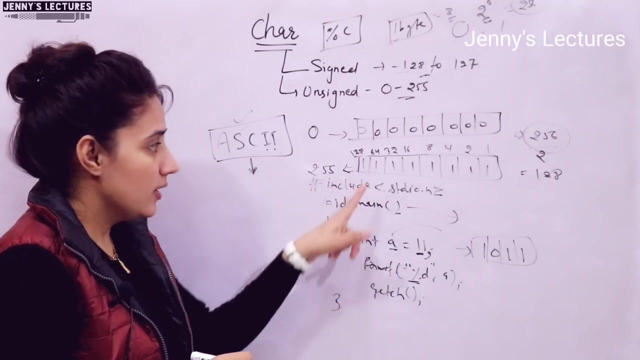 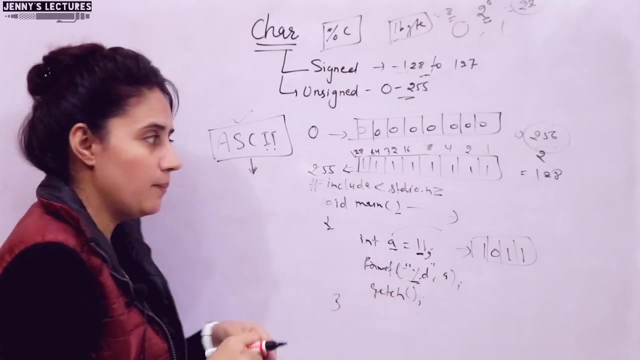 to store characters or to store any text into computer or any telecommunication devices. you right, and here we have codes for every alphabet, like in english. we have small letters, we have capital letters, numbers from zero to nine and some special characters, like some special symbol: hash, this symbol, this symbol, equal to the symbol for these we have numbers, like for a, the value would: 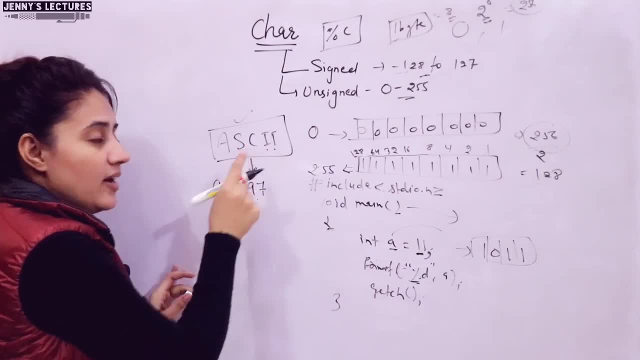 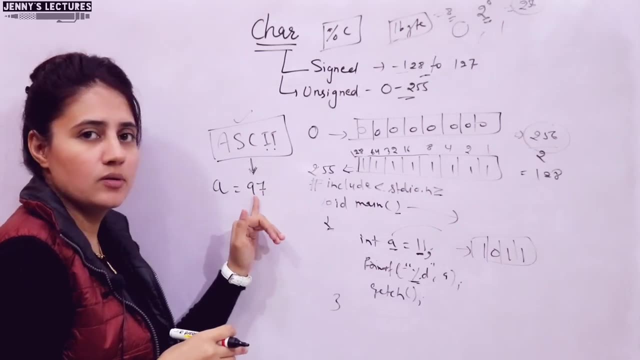 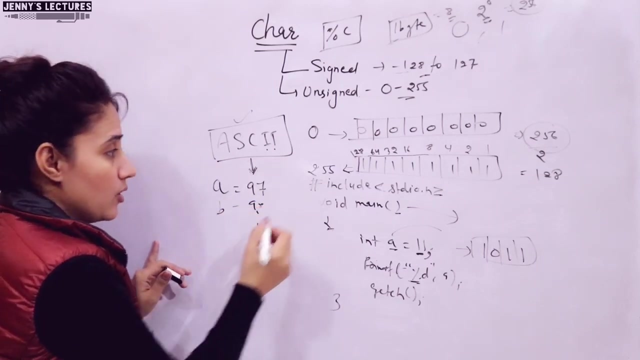 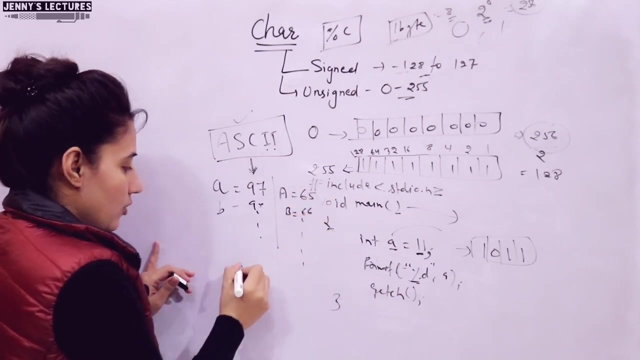 be 97, the code is 97 and this is what standard code. you cannot change this value. americans, they decided that a would be stored, a would be converted. the sky value of a is 97, small a like this, b 98, and so on. for capital a it's 65, for capital b 66, and so on. zero to nine. they are also having their own. 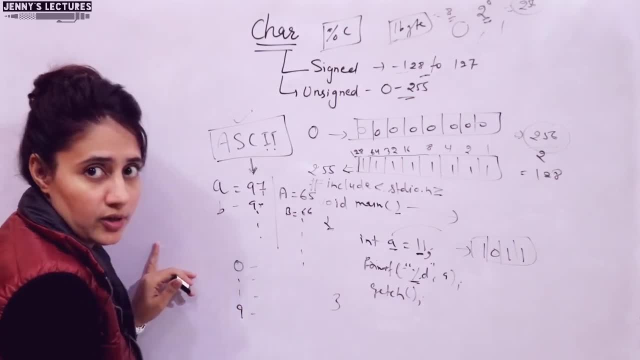 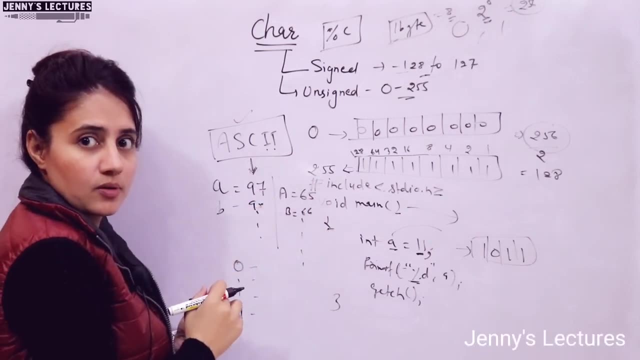 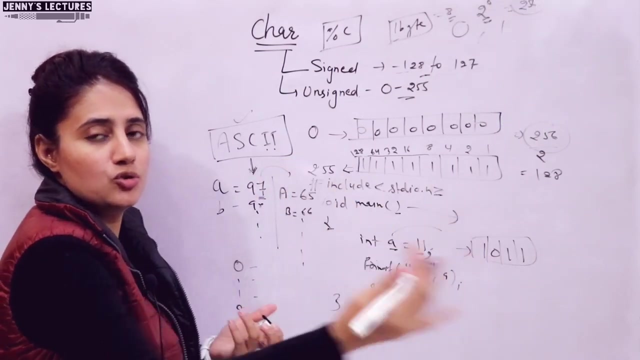 number from 48 to, like this, 48, 49, like this. special characters are also having their own corresponding these numbers. right now, a is 97. now this would be converted into zeros and ones and that is going to be stored in computer memory directly. we cannot store a in memory, right? that is why. 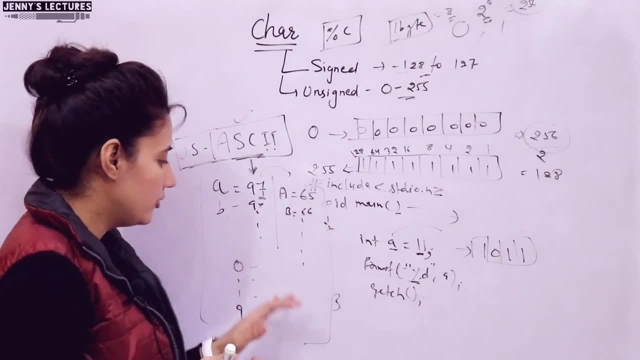 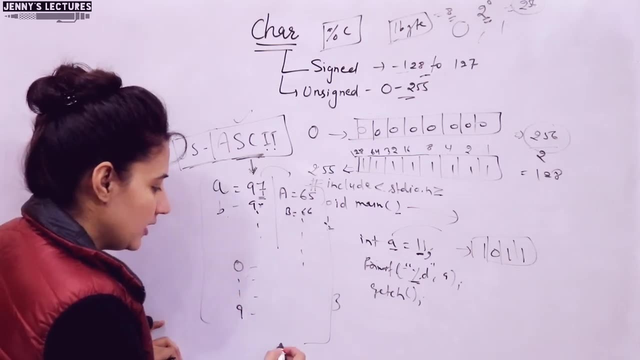 we need character system now why they have given code for only 256 characters. if you combine this- small letters, capital letters, zero to nine and some special symbols- then definitely the number would be less than 255 or less than 256.. that is why they have given code for. 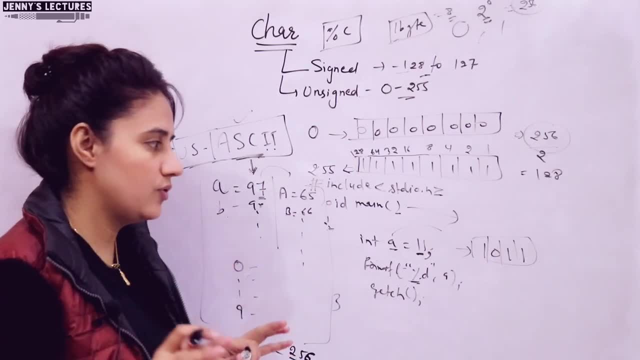 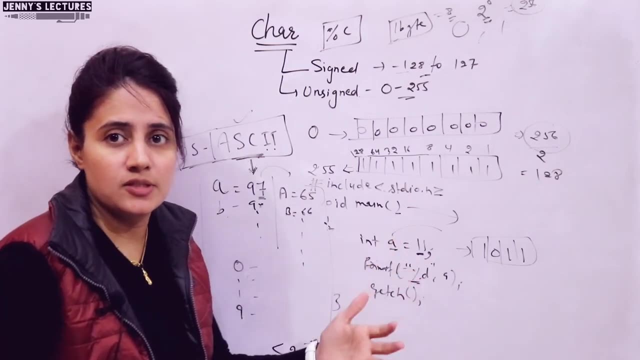 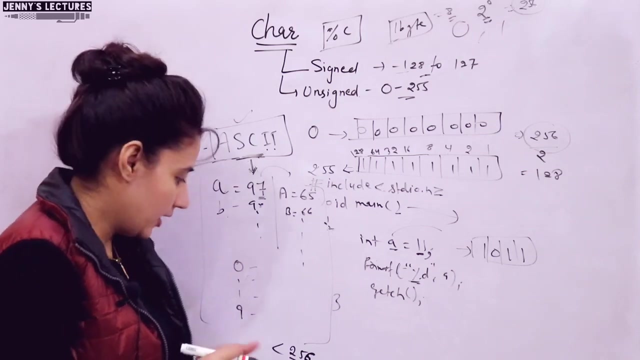 from for 256 characters, from 0 to 255. 256 you can say symbols, characters and symbols. many modern encoding system are also their character system that are based on sky only, but they include additional characters also. right like here, we have only 256, maybe some. 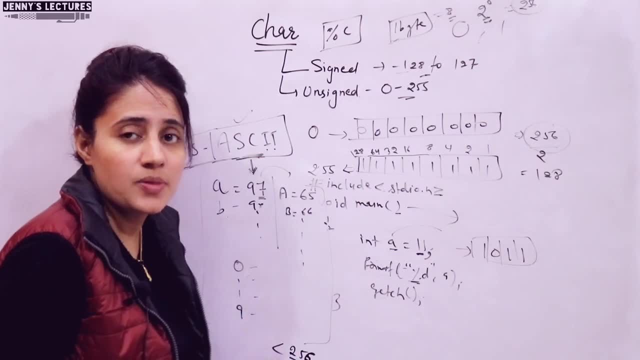 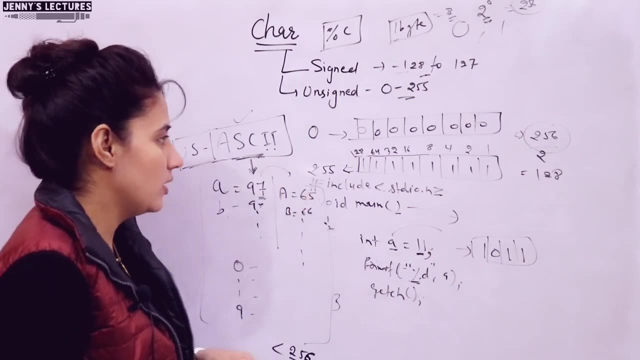 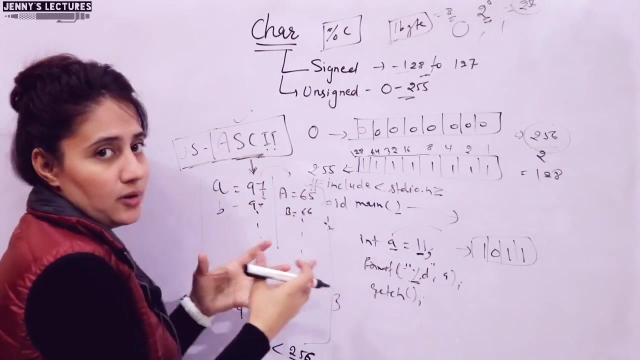 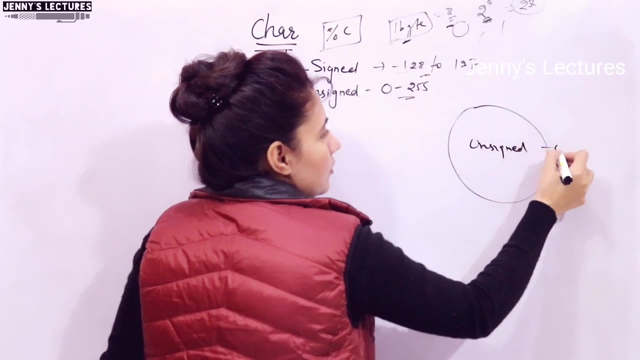 other encoding system, that another character system that is having these codes for 260 symbols, for 270 symbols, but that is based on sky only. right now let us discuss with the program what output you will get if you use these characters and these numbers in our program. we will discuss with the help of a program. now, this is, for suppose, unsigned. 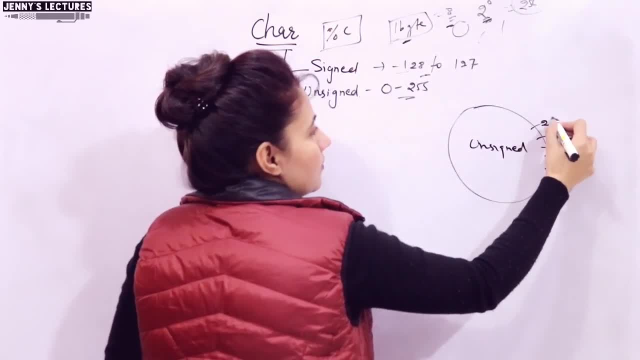 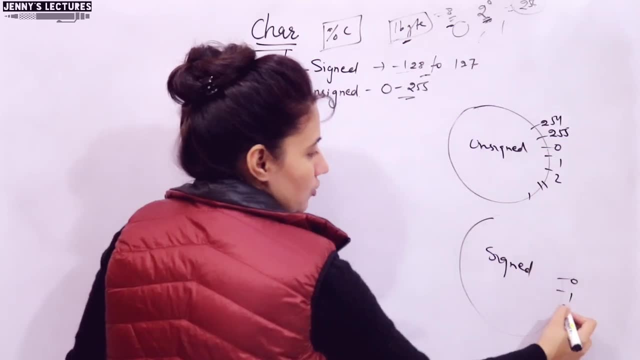 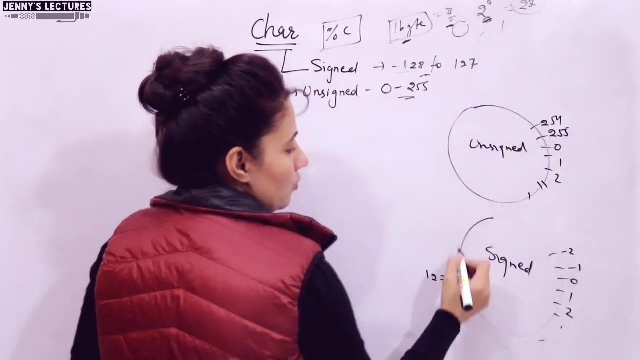 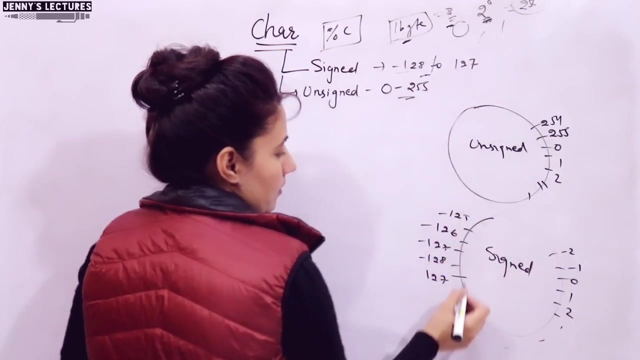 from 0 to 255, like this, and this is for signed char, 0 to 255.. here, clockwise, we have positive values till 127 and here we have minus 1, minus 2, anti clockwise till minus 128. right, these values we have now suppose. if i print, see please. 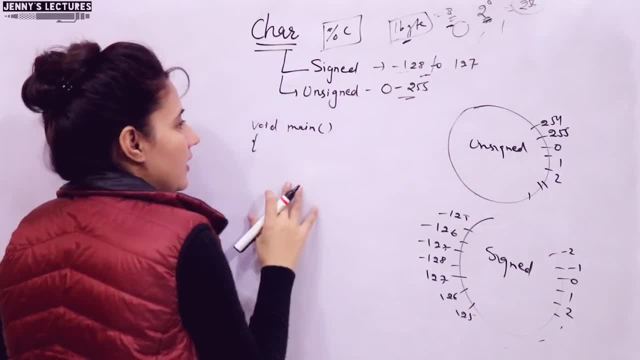 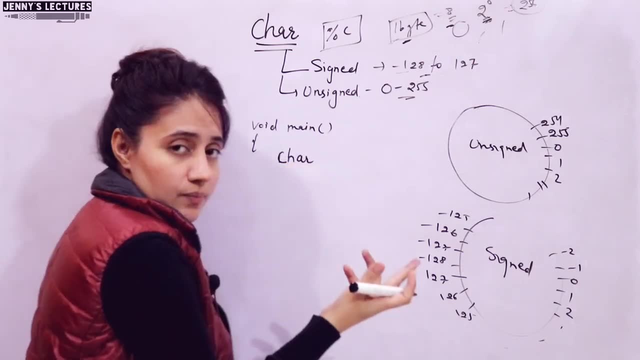 include those header files also. i am not writing header files again and again every time, but you have to include. suppose i am the, that data type is char. here we will. uh, we will take a variable name. you can take any variable name: a, b, c, c, h, anything. it's up to you, i am. 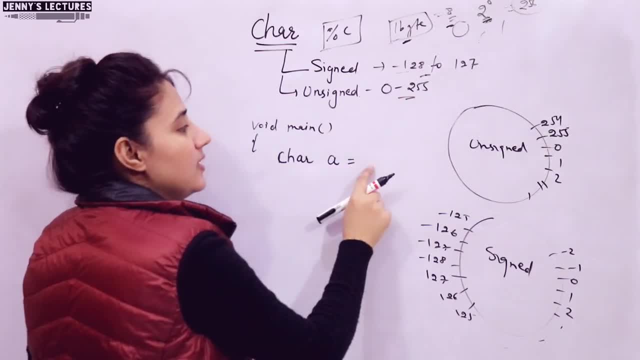 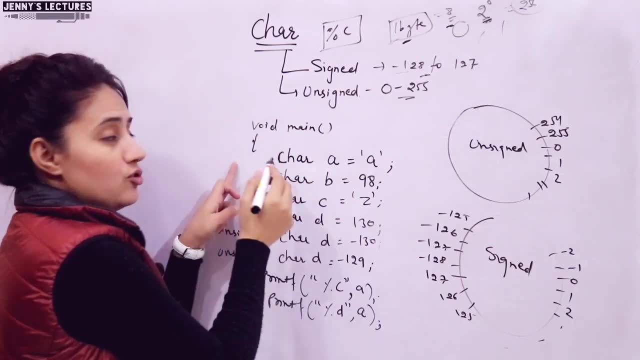 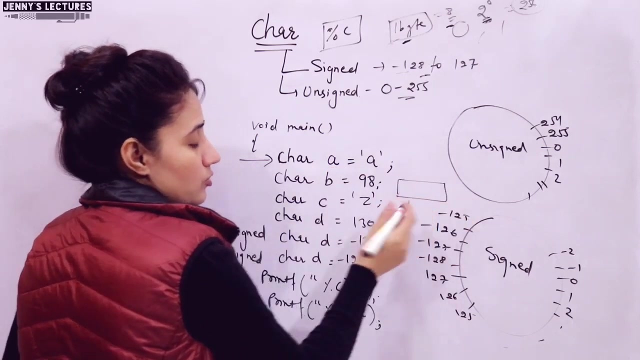 taking suppose a and the character. suppose i am initializing it with this one. now suppose i am taking this program. first of all, take this line. the control will go the first line of main when we execute a program. now. char a, so value would be assigned to so, so memory. 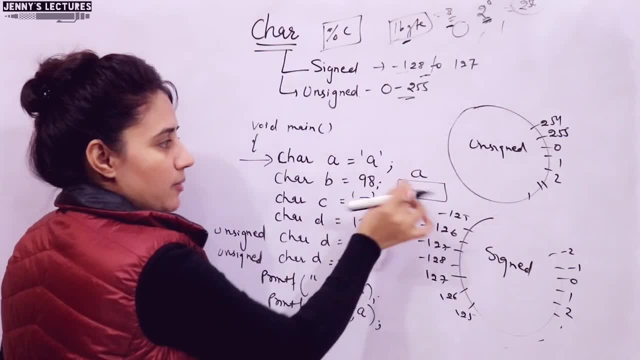 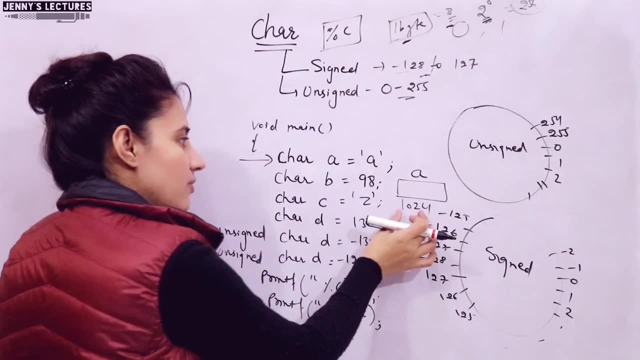 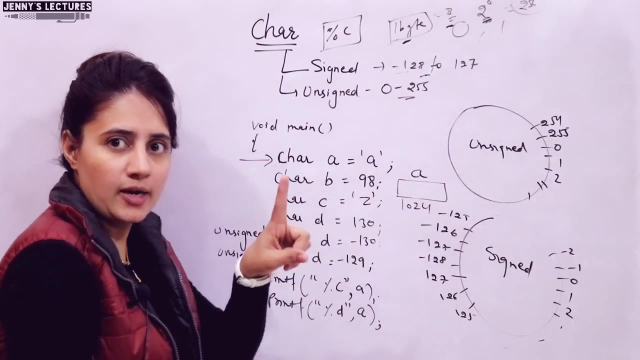 would be assigned to variable name is a. some memory would be assigned and suppose, uh, the address is 1024, i don't know the address. i am just supposing address is 1024 and the name of this memory location is a. now here it is what. here we can store one byte eight. 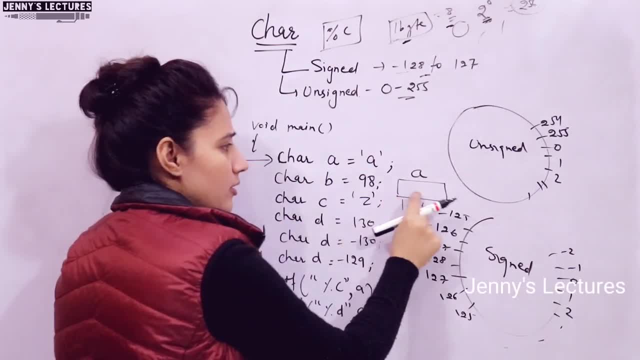 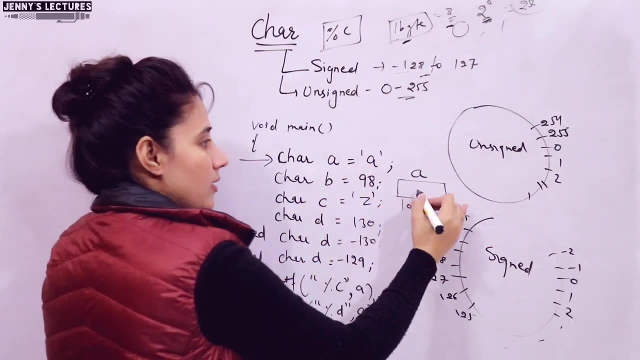 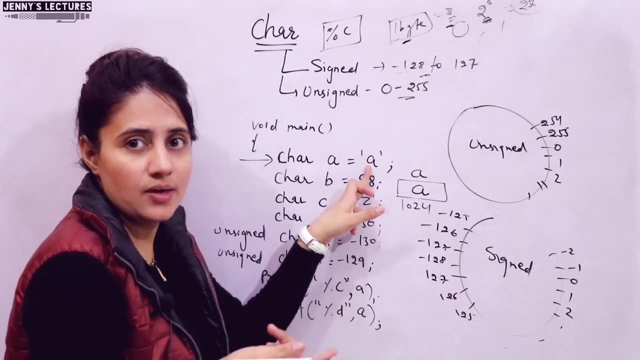 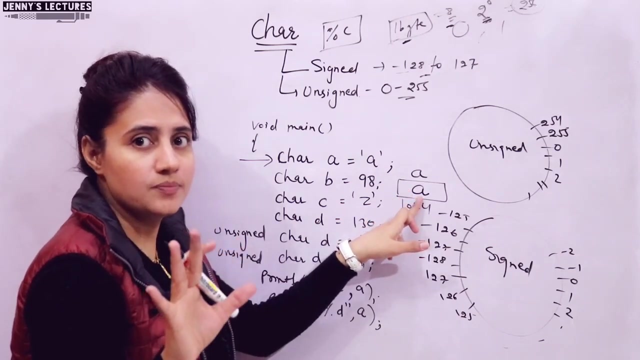 bits, data right now, what you are going to store here, initialization is a, so this is what a character. so here i am writing, a- would be stored. but here what would be stored? corresponding to a, the value is 97.. okay, 97 and 97 in binary form, zeros and one, one form that would be stored here. right, i hope. 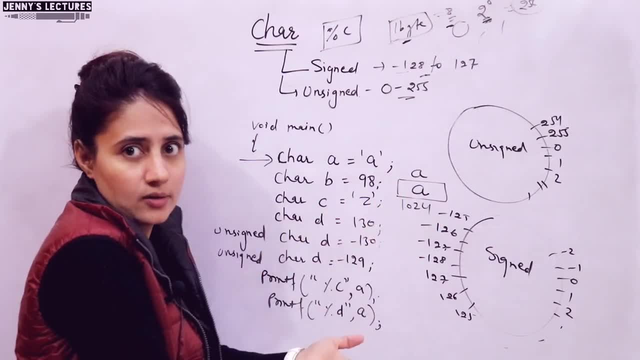 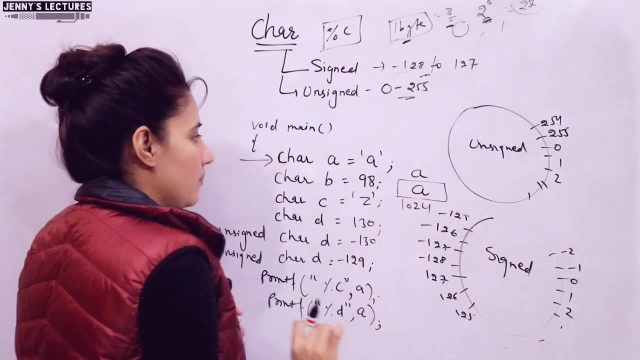 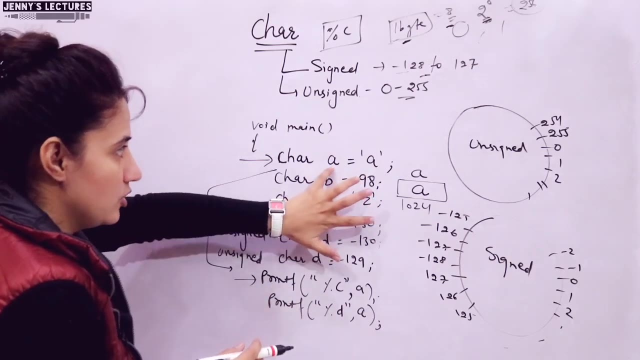 you are getting my point, because in memory obviously we cannot store any character. so 97, 97 convert into binary number. that would be stored here. but just for understanding purpose i am writing here a only now, when you print with percentage c printf. these we will discuss. uh, after this, this statement, suppose here we have only one statement in. 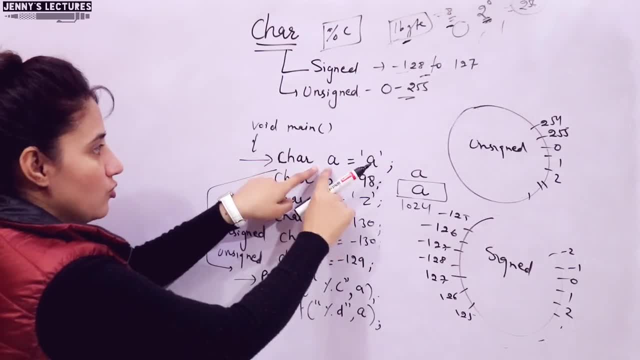 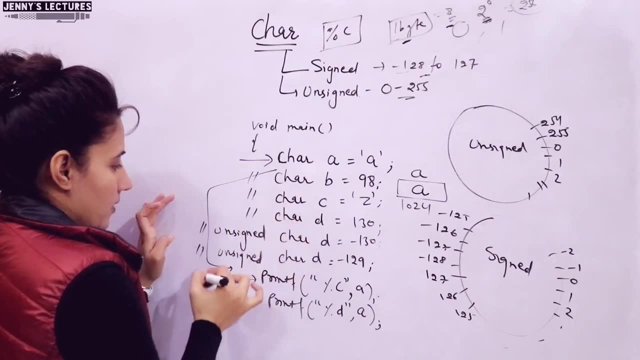 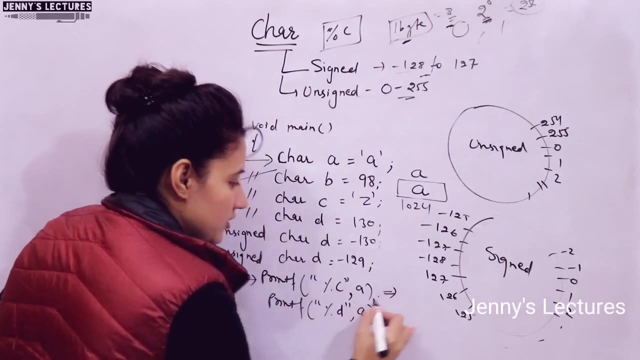 program and then we have this statement right. so now control will go directly to printf. we are not having these statements. if i suppose right here, comment this, this one. this is single line comment, so these lines would be completely ignored by compiler right now. what would be the output of this thing? 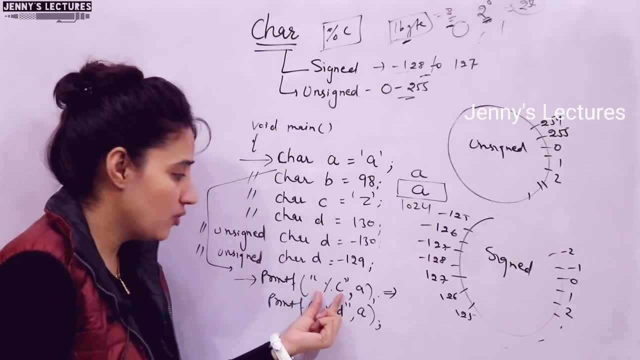 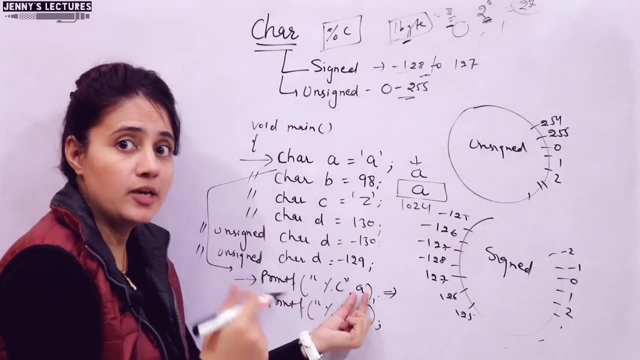 percentage. c means compiler will come to know this format specifier is what for character means he has to print a character from where it will print character. now see what is here. name a: Now it will check that named memory location A From memory it is going to fetch the data. 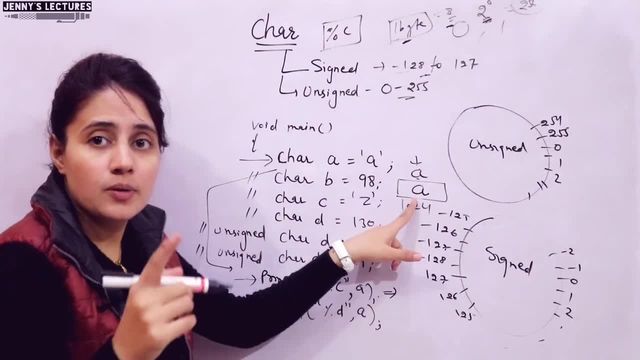 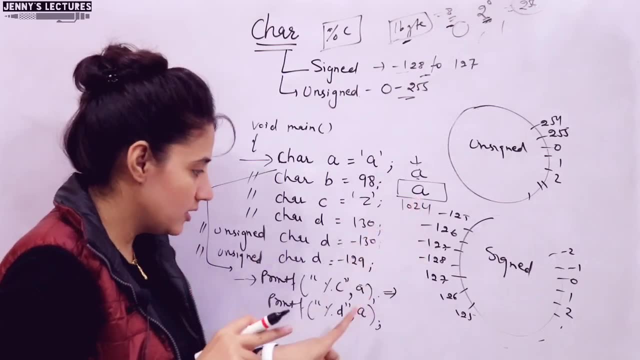 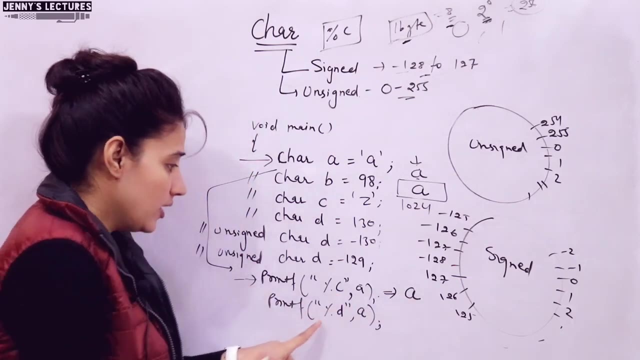 Now at A, what we will have? binary number corresponding to 97. And 97 means A, because he has to print a character, So that is why it will output will be A only Right Now. next comes to this one Suppose you are printing A with percentage D. 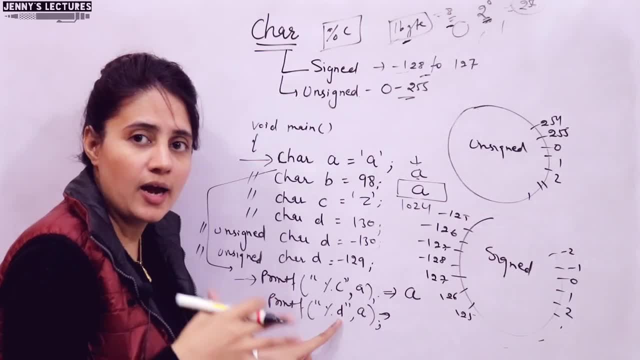 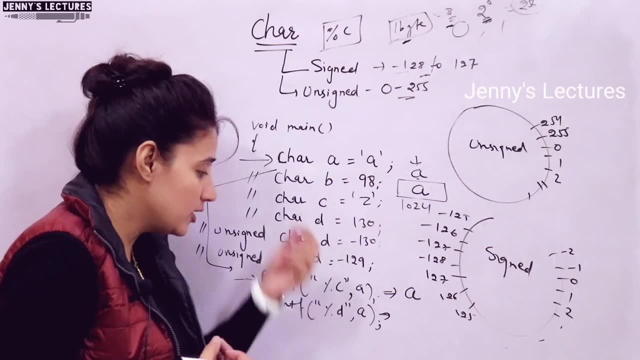 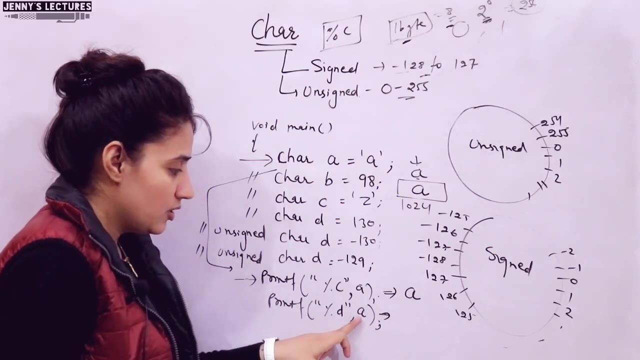 It means percentage D means compiler will know the meaning of percentage D. That is, he has to print integer value. This format specifier is for what Integer? It is not for character. Now it will print integer value. What is going to store? 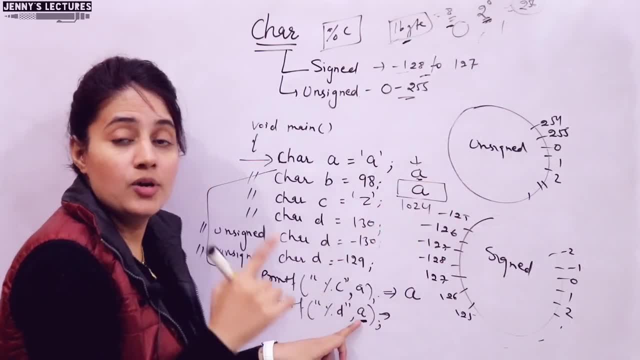 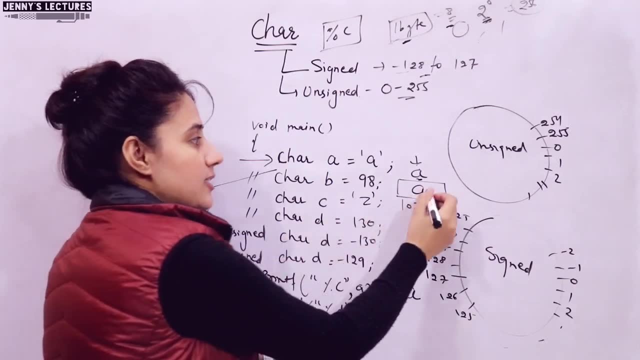 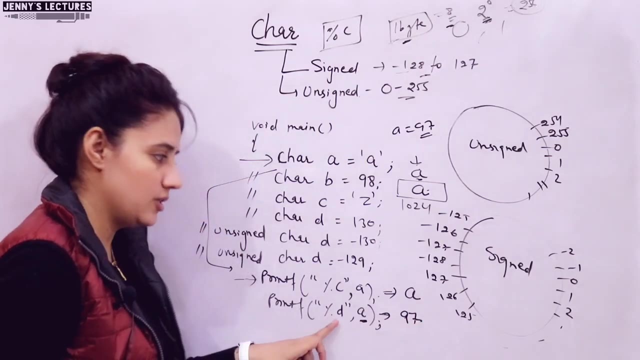 Whatever value is stored in this variable A. Now in A we have stored binary, binary number, binary form, of which one 97.. 97 because small a is in a sky code 97. So it will print now 97 with percentage D. 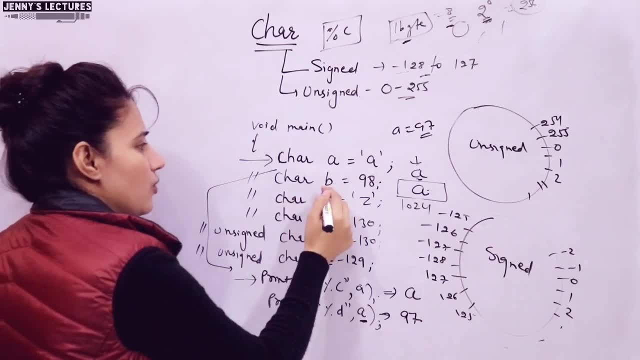 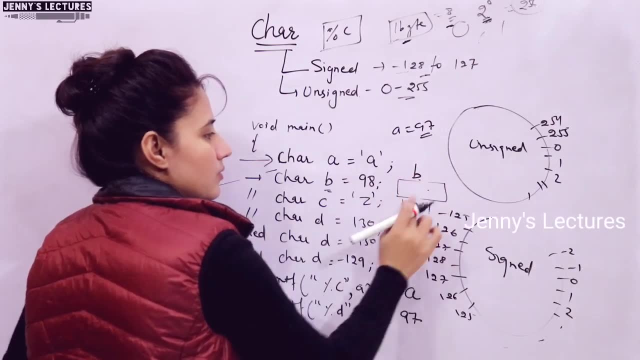 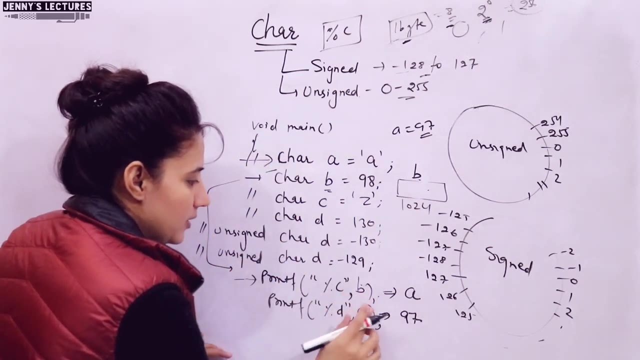 I hope you are getting my point. Now let us take this one. We have character B and 98 and this location is suppose B now, And address is this one, or you can change the address. Now this line is comment line And here I am printing B and B. 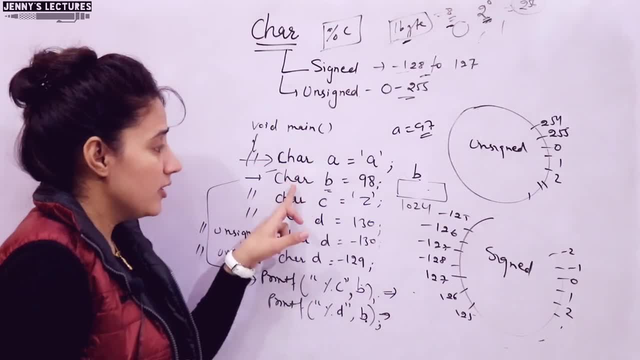 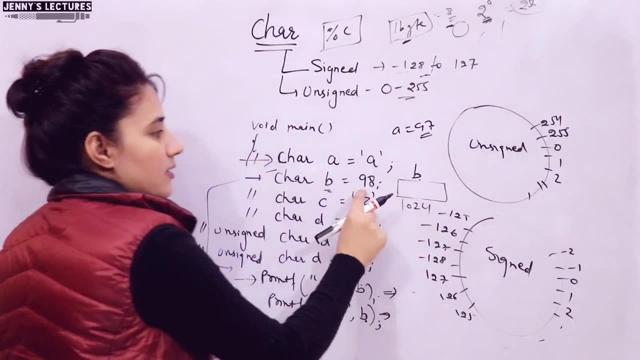 Now what would be the output? See Character B, See by default character. I am taking no signed and unsigned. I have written, So it is what Signed. Now, when we will store this 98.. First of all, obviously we have to check it is within the range or not, right? 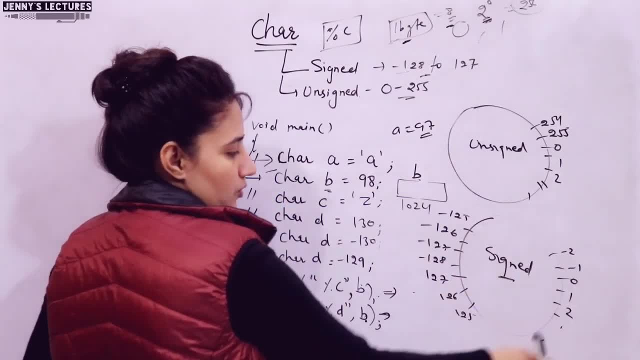 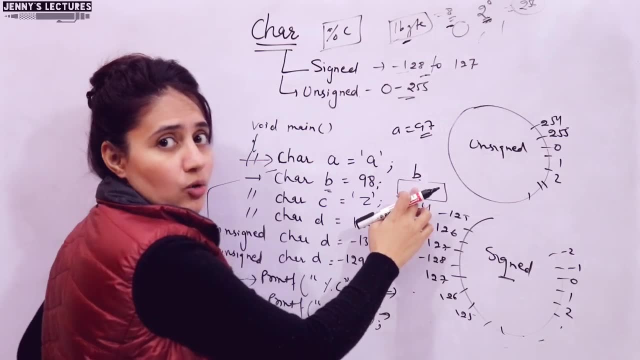 So it is for signed. Go to that signed circle. In signed circle we have 98 or not. Yes, we have 98 is within this range Less than 128.. So here, what would be stored? The corresponding binary value of 98.. 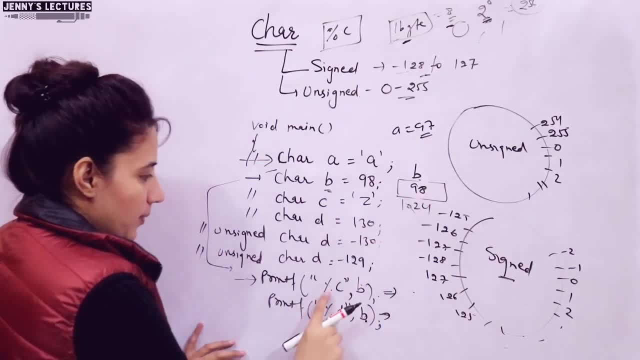 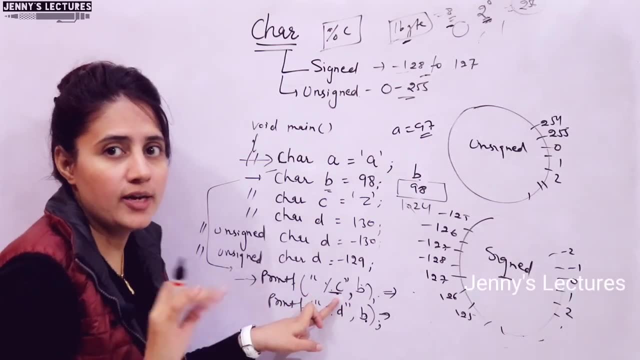 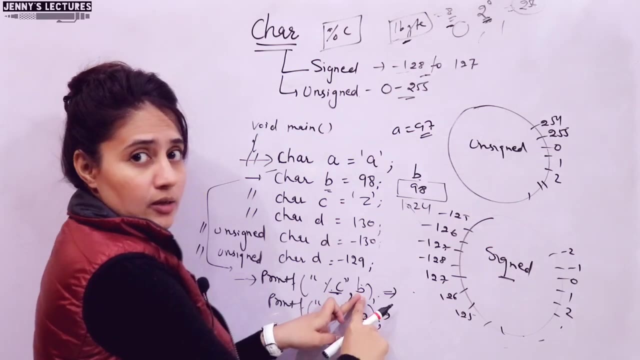 Because here but here I am writing only 98.. Now, when we are printing with percentage C, then percentage C means compiler has to print a character, not an integer value. because this format specifier is for for what? for character, right Now, corresponding to B, the memory, the data it will fetch from this one B. the name of that memory location is B. 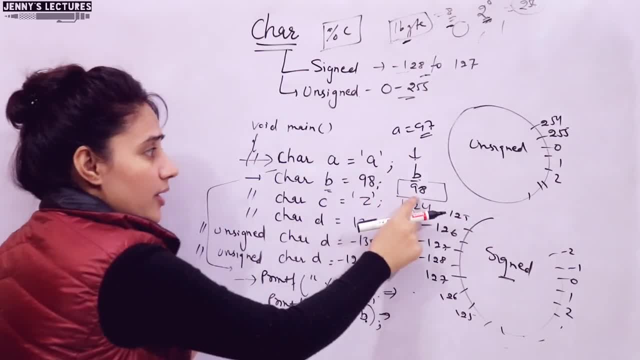 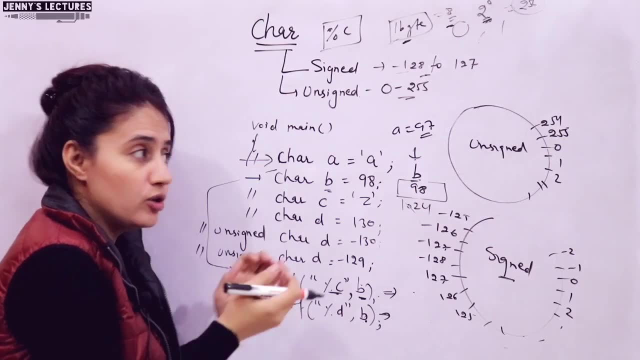 So here it will fetch data from here. Now, here we have 98. that binary is in the form of 98. But he has to print a character. So now, corresponding to 98, the character is what? B, small b. So it will print small b. 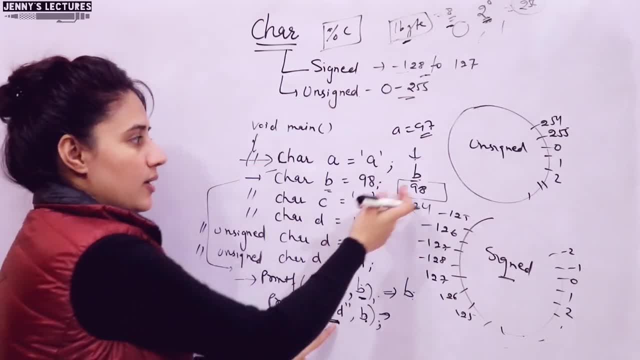 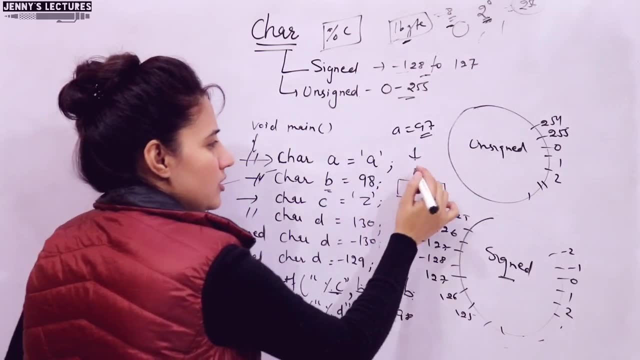 Here we have percentage D. It has to print integer, So it will directly print 98. Now let us take this one Percentage C. Now this is comment line. Now, this is suppose C and memory location. I'm not going to change that as same, or you can change it. 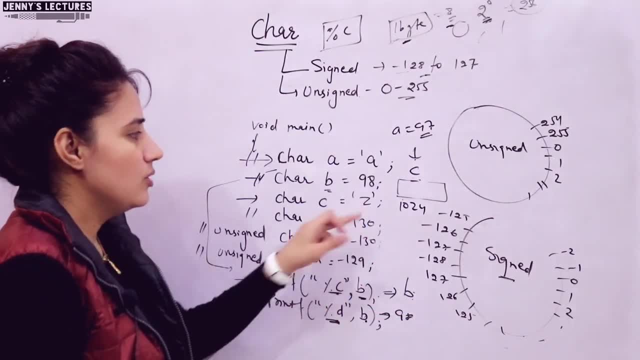 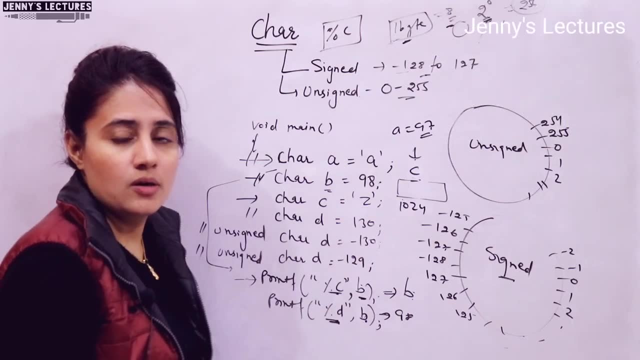 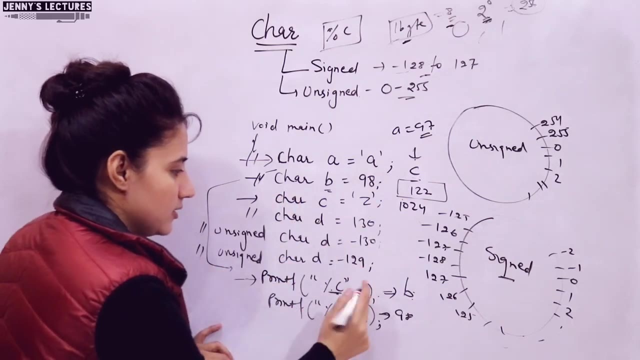 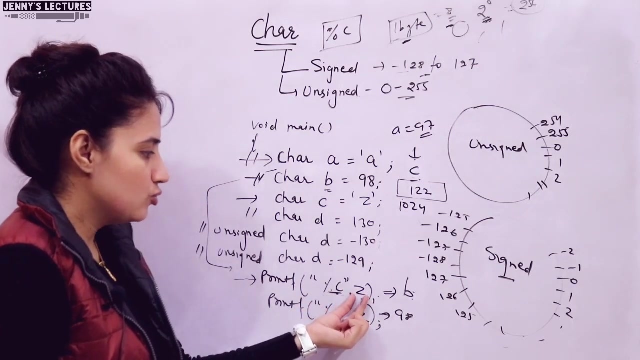 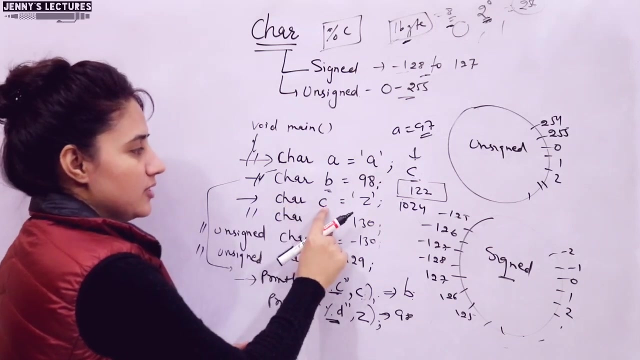 This is just an example. Now here I want to store Z Now at this place, rather than Z. what is going to store? Z means, I think, 122. So here 122, binary form of 122, is going to store. now, when you will print Z here, what would be the output percentage? C means it has to print a character now from where it is going to store what value it has to print from this C. sorry, here I will print C. the name of variable is C, not Z. the value I'm going to store that is Z. 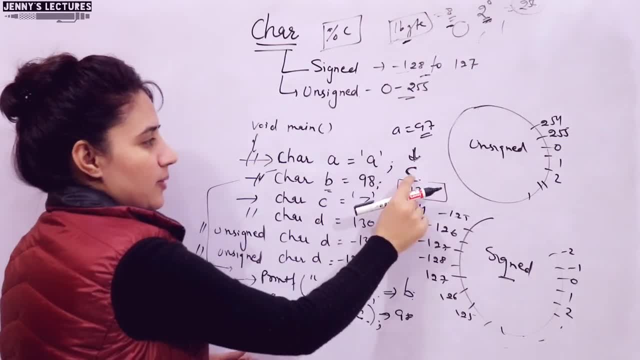 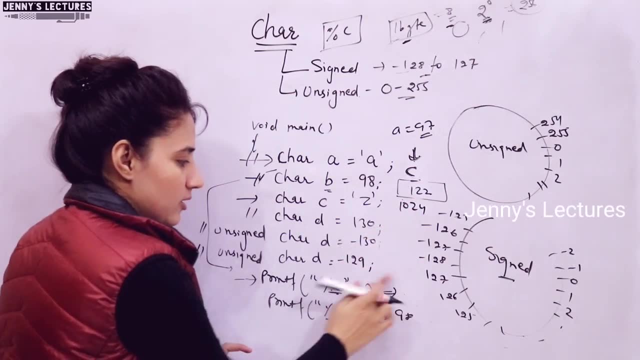 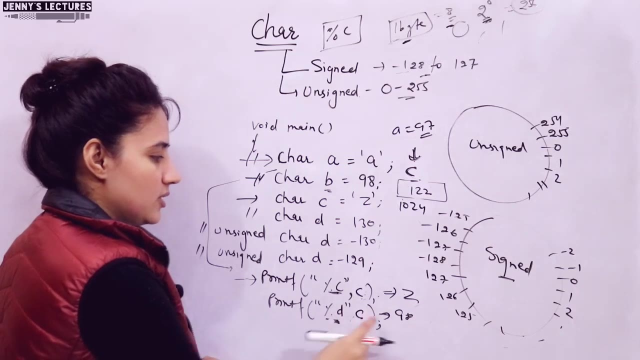 C. So from here, this variable, this memory location, it is going to fetch. But here we have what 122? binary form of 122. So it will print corresponding character for this 122, that is Z. And if you print with percentage D, then it will print 122 only because it is for integer. 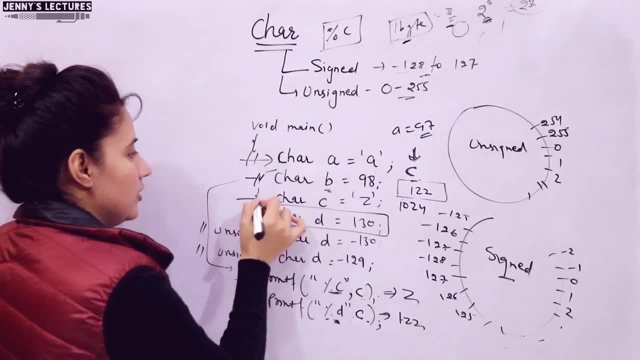 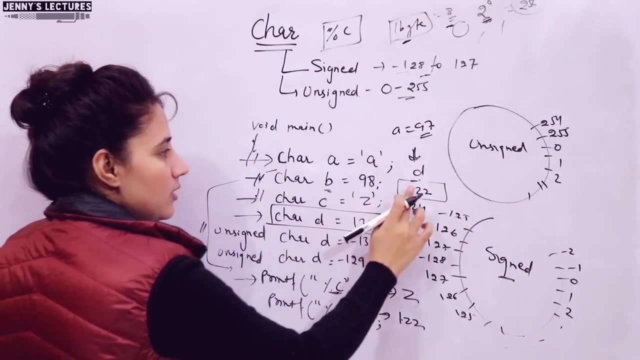 Right now this one. what about this one? This is comment line now. Now I want to take this one. Control will go here. Suppose a memory location would be Allocated to variable name is D and the address is this one only. 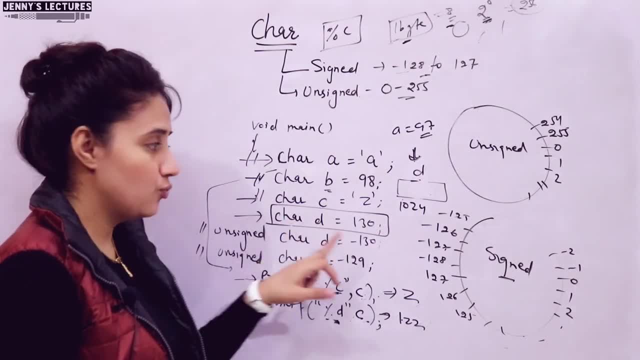 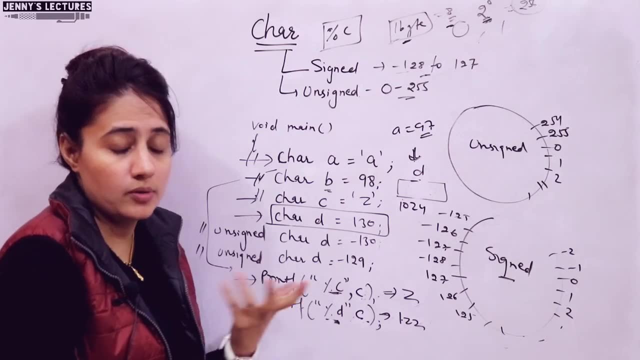 Now I want to store here 130.. This is what signed care value is 130.. It is not within this range. Now, what is going to store? What value is to be stored here? It will not give out error. It is not syntax error. 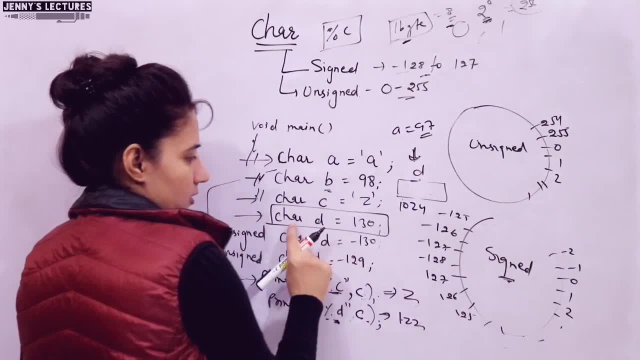 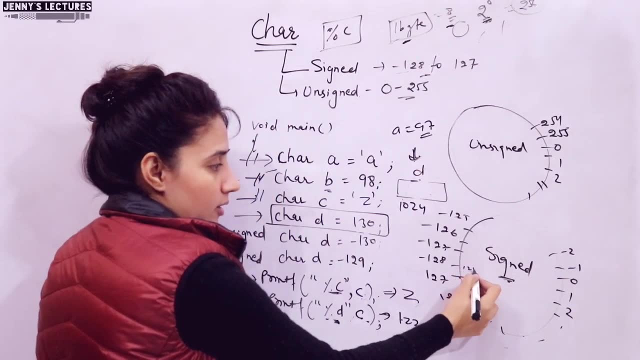 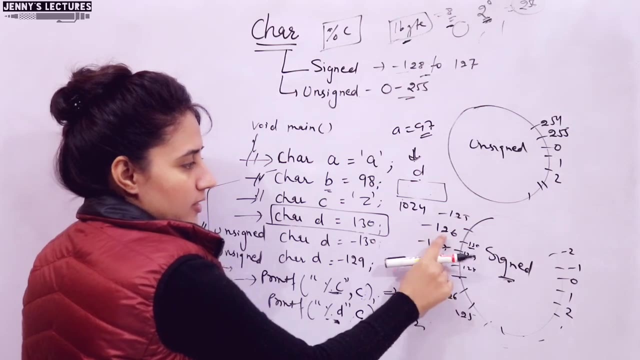 Right now, see the circle- the sign circle, because it is signed care- where you have 130, 0 to 127,, 128,, 129, 130.. Corresponding to 130, what we have the value is minus 126.. 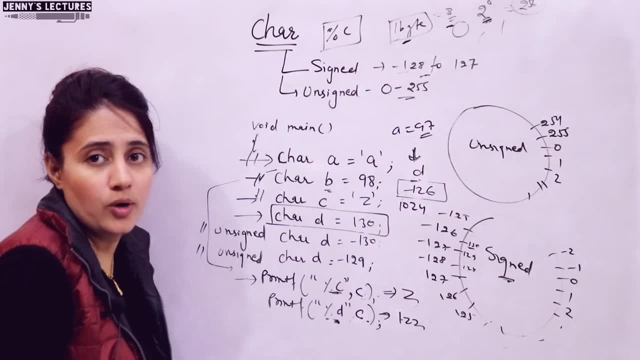 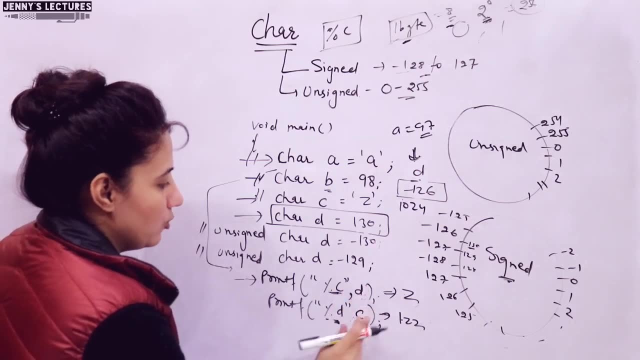 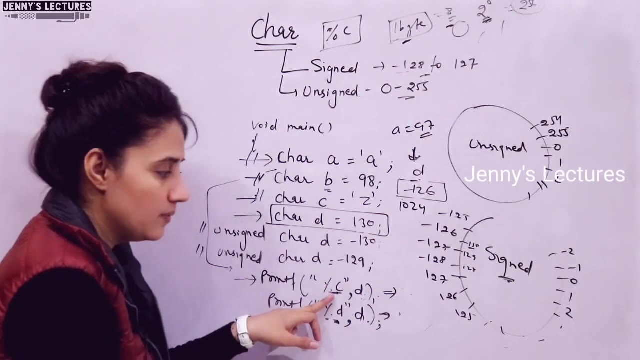 So that value would be stored here Minus 126, corresponding to this 130.. Now when you will print with percentage C here I'm going to print D and I'm going to print D. So now, when you will print with percentage C means it has to print a character from where it is going to fetch from. D name is here. 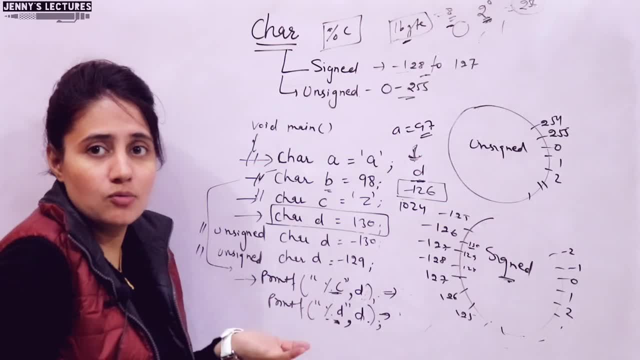 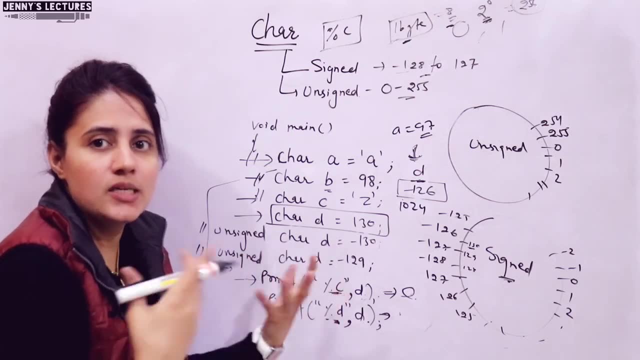 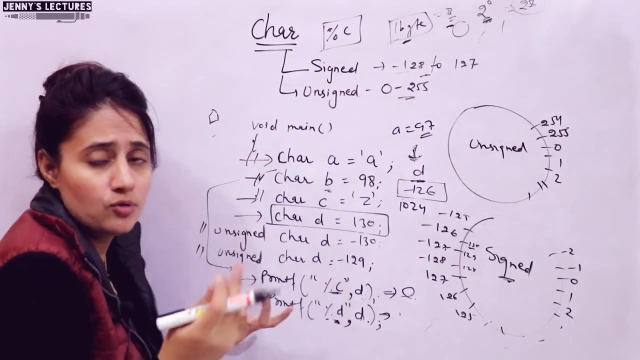 Now with this minus 126.. What is that corresponding character? any garbage character. it will print here any garbage symbol, not character. any symbol. Sometimes it may print like this kind of symbol. It may print any symbol Like: maybe you can check out in your compiler when you will run what symbol it will print, right. 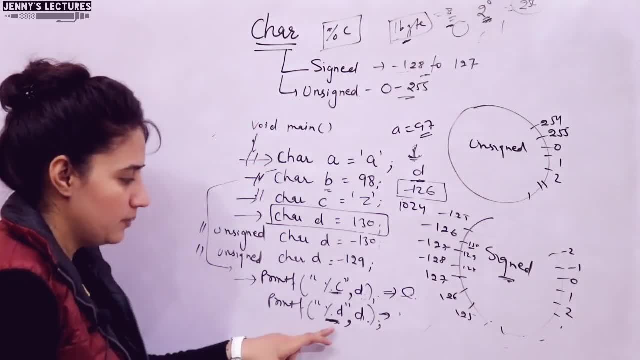 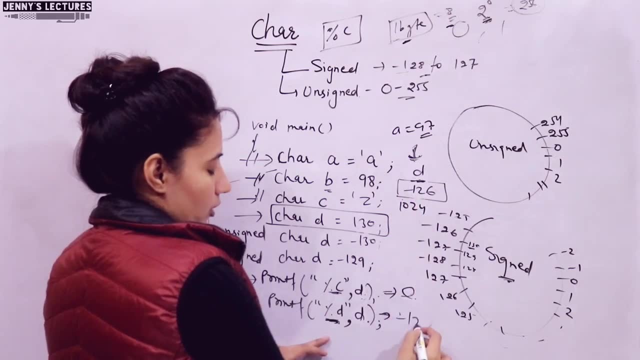 It will not give error. Now, when you will print with percentage D, it means it has to print an integer right Now. what it will print? it will print directly minus 126.. Because, see, it is for signed. percentage D is for signed na percentage U is for unsigned. 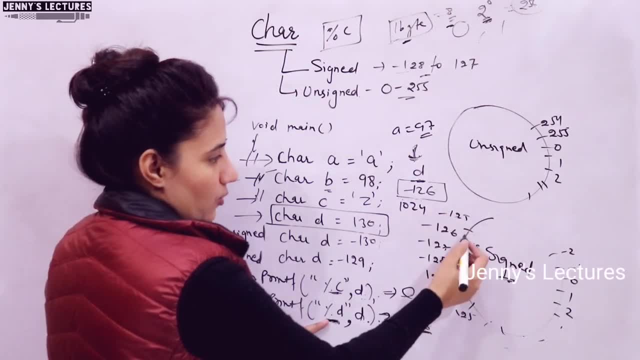 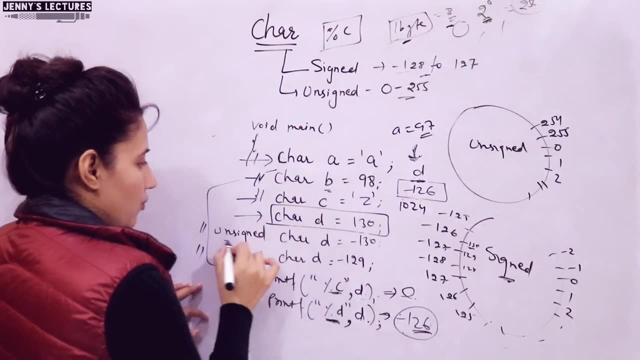 So in signed do we have this minus 126?? Yes, we have minus 126.. So it will print this minus 126 here Right Now, suppose this one now with this one it is unsigned char, but here I'm storing minus 130. 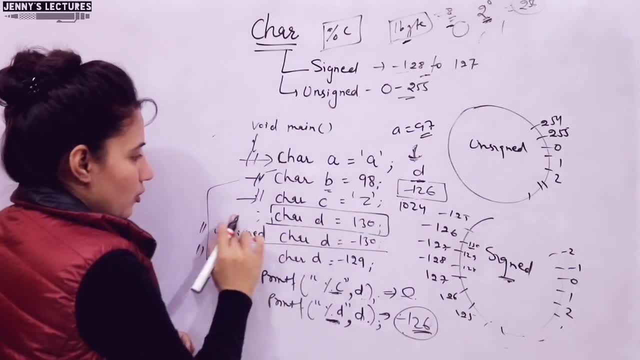 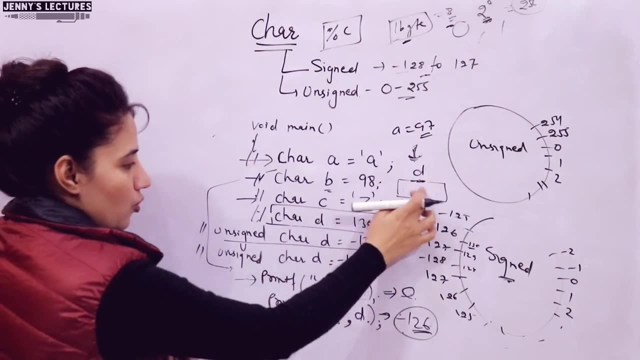 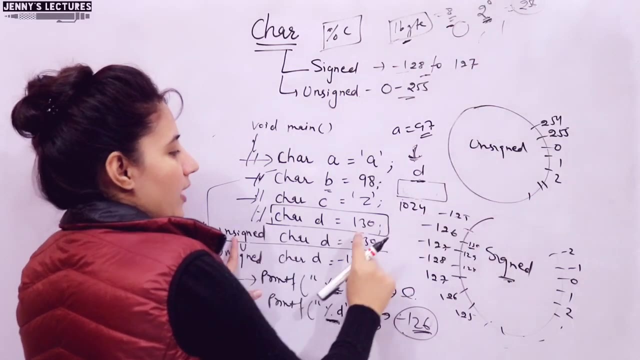 Then what would be that result? Let us suppose I'm going to comment this line right, And that same variable name I'm taking here D. So here what would be stored here? Unsigned char value is minus 130.. So in unsigned check, where is this one, this value minus 130. 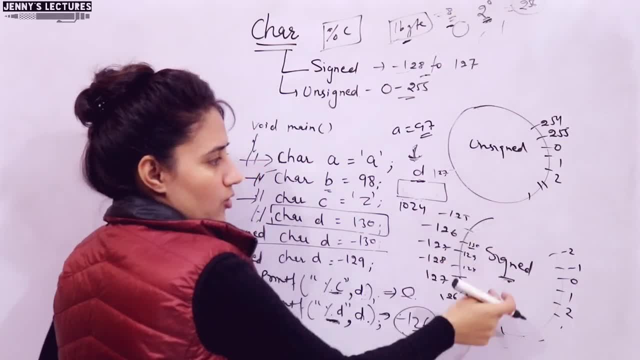 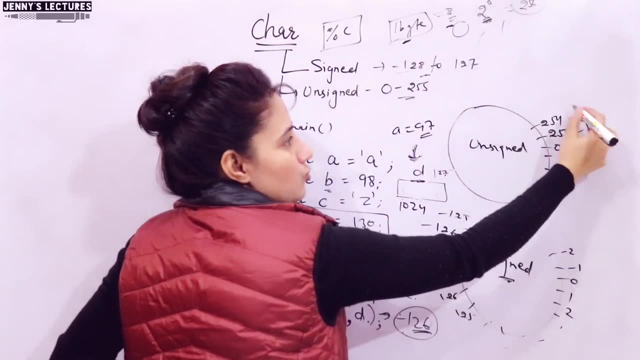 Here somewhere we will have 127, because these are somewhat same. Here we have positive value, Negative value. if you will write corresponding negative value, then minus 1,, minus 2,, minus 3,, 250,, 3.. Like this: 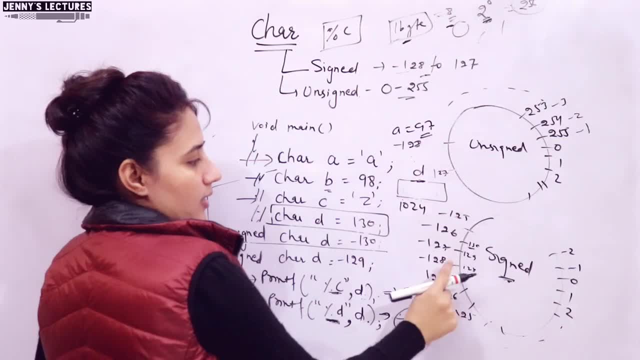 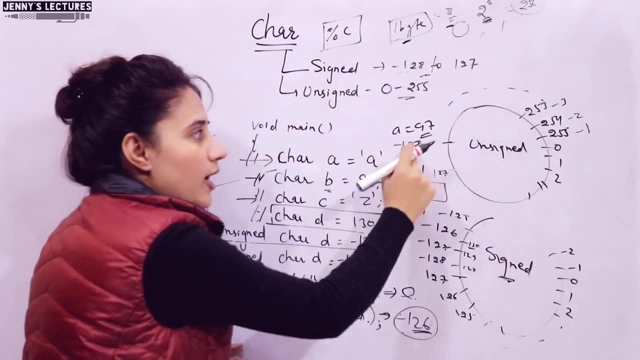 And somewhere we will have a value, Negative value, minus 128, like in this. we have right, But here actual data would be plus data, plus value only, But corresponding to that we have minus 128.. You can see in the circle. 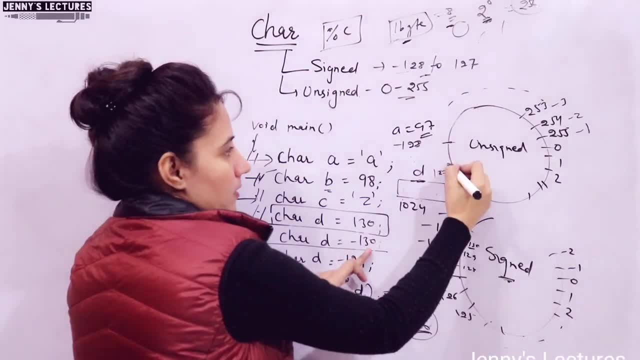 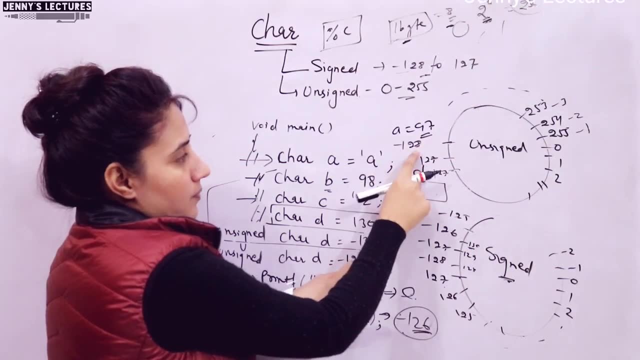 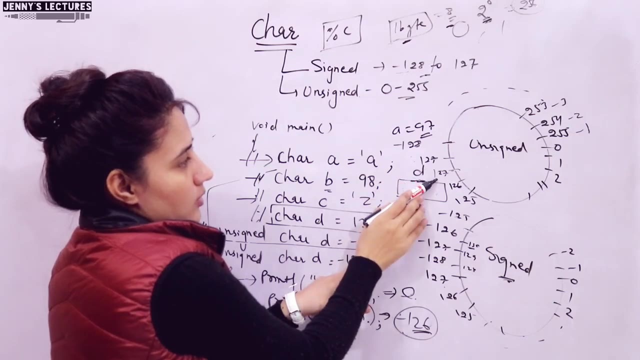 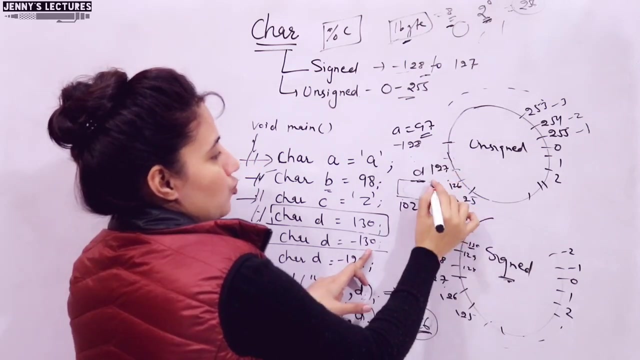 Now where this minus 130 will lie. here, At some place we will have 127, also right, Minus 128. Then here we will have 126, 125.. Minus 129, minus 130.. So minus 130 means here we have 127, this is 126, 125, 124, like this. 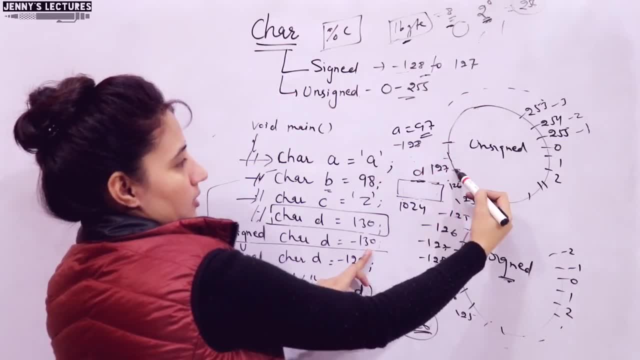 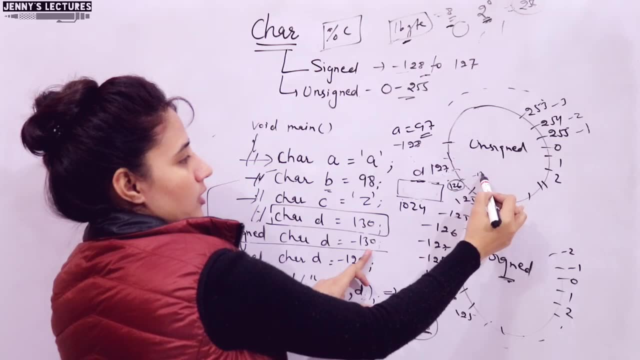 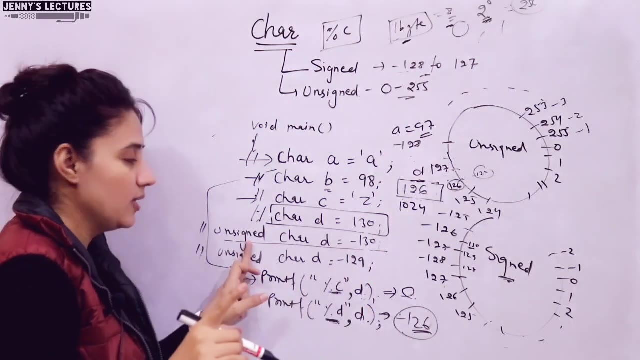 So minus 128, then if you come this side, minus 129, minus 130. So corresponding to 126 minus 130, value is there. So what value is to be stored here? 126, right, Because here I'm taking unsigned. 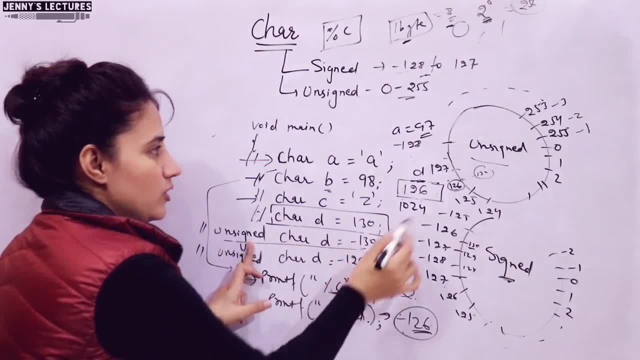 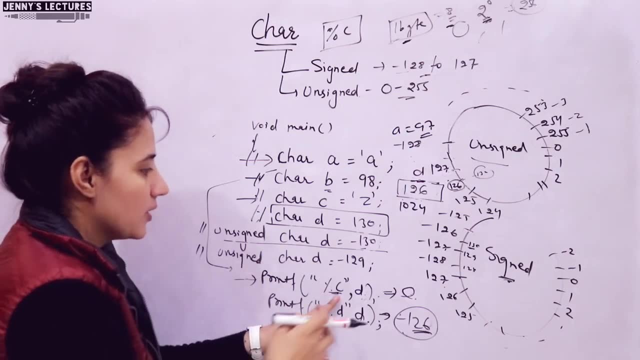 So unsigned circle, I'm going to write Refer Corresponding to minus 130,. what value is there in unsigned circle That would be stored? The binary form of that value would be stored. Now, when you will print with percentage C, then character value of 126 is what. 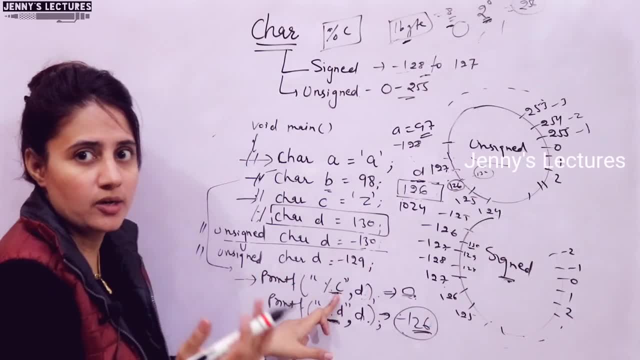 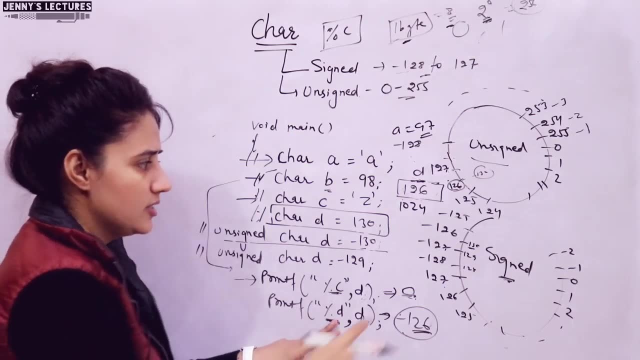 Whatever character value That would be print. That would be the output. You can check Right And with percentage D it is for signed one In signed Now, when we will print. it is for percentage D. format specifier is for what? 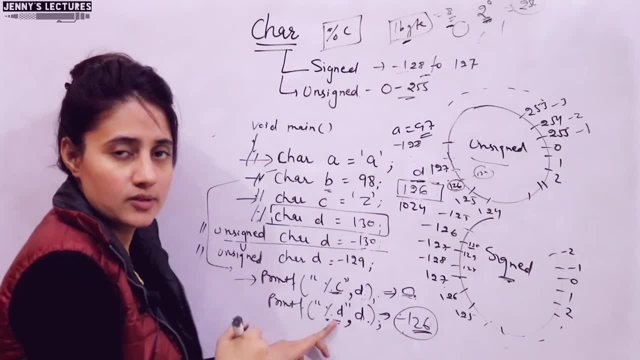 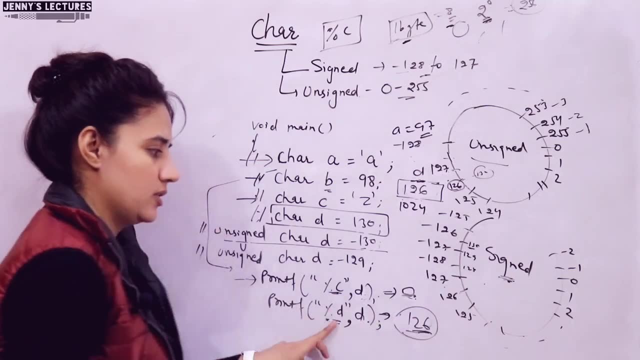 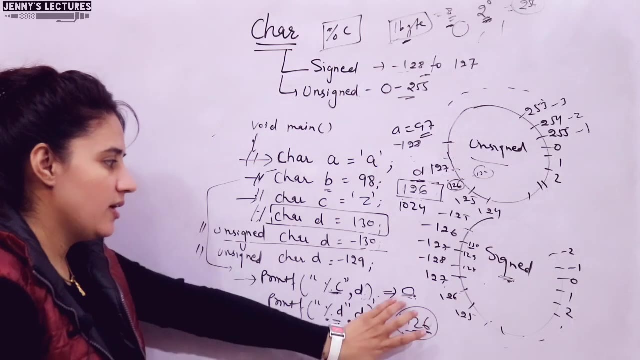 It is for signed integer, Signed value. So it will refer this circle. here We have 126.. Yes, we have 126.. So it will print plus 126 here. So you are initializing with minus 130, but actual value is 126 and some corresponding. 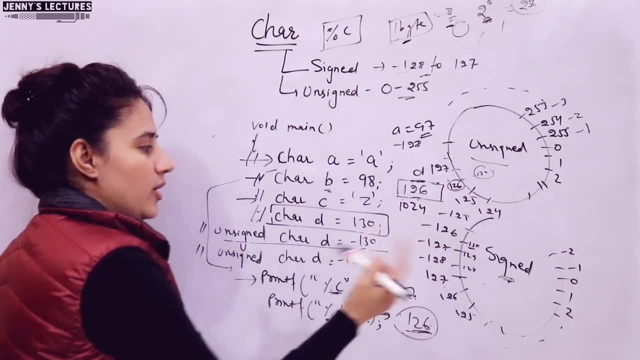 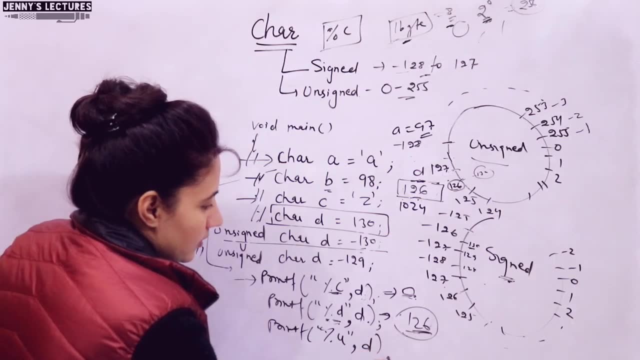 character to this one, because actual value that is to be stored in this is 126, not minus 130. And if you will print it with, suppose, percentage U, then what would be the output? percentage U means Unsigned, So it will refer this circle unsigned. 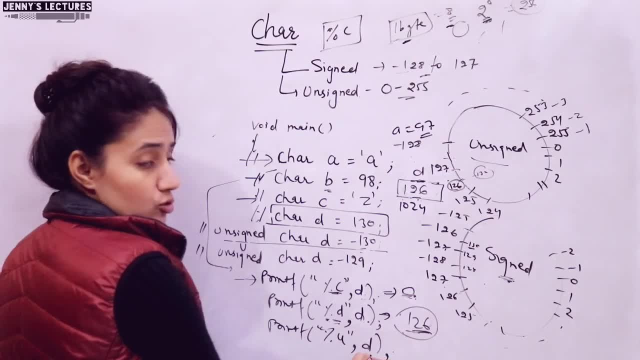 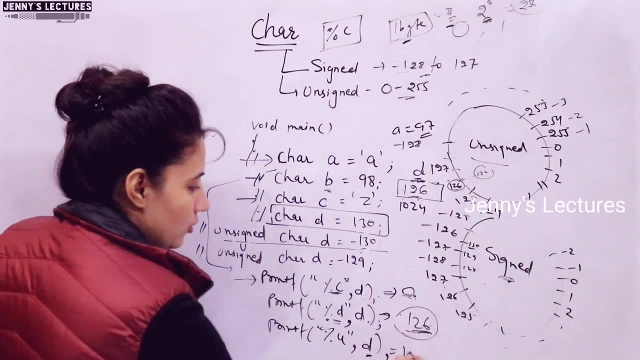 And now in unsigned the value in D. from where it will? it is going to fetch value from D, this memory location. Here we have 126. So check out in unsigned We have 126.. Yes, we have. So it will print 126 only. 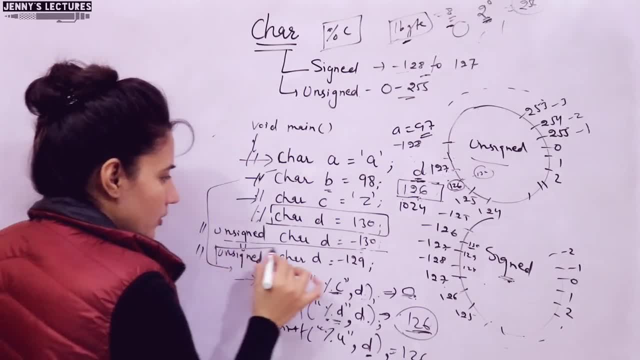 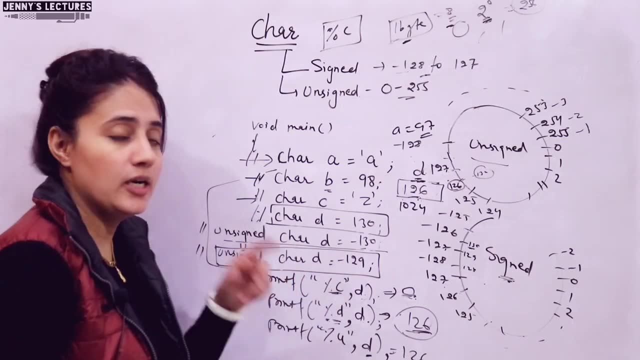 In both cases it will print 126.. Now, in this case, what should be the output? you have to tell me in comment box If I write this line: unsigned char name of variable is D and I am assigning minus 129 value. So now you dry run. 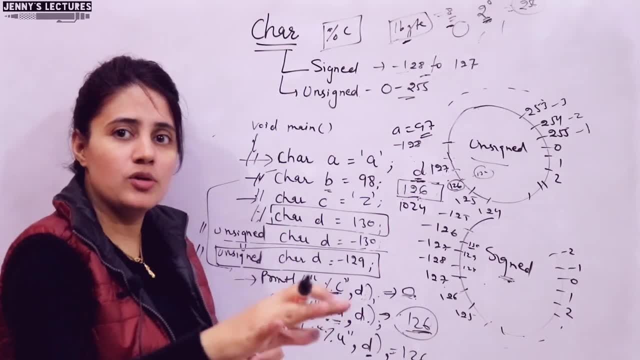 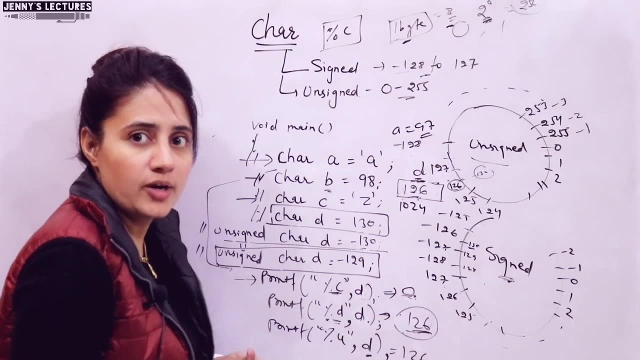 First of all, this program. it is not that you just directly write down on your system and check the output. No, Be honest, Dry, run this program using these circles and then check what is the output And then after that you can tell your answer with your system. because if you want to be, 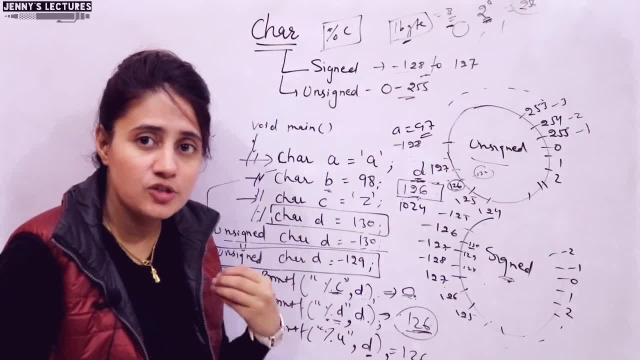 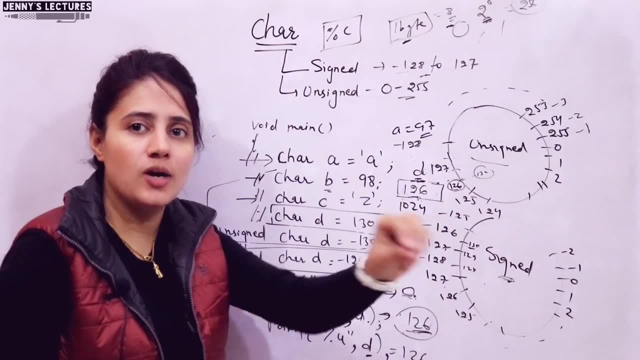 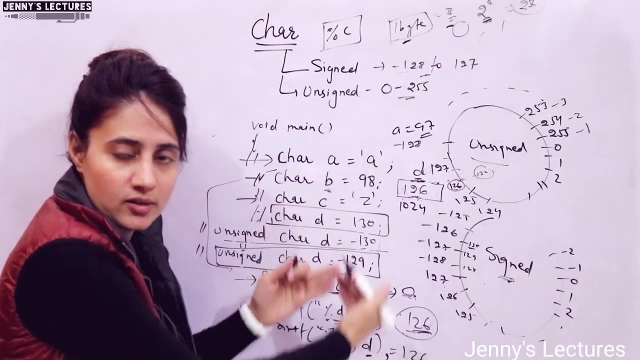 very good in programming, then definitely you should. First of all, you make a habit of dry running of that program directly. Do not just skip, Do not just jump to your laptop. write program. If it is a simple program, Then also write program on pen and paper. dry run that program, check the output. 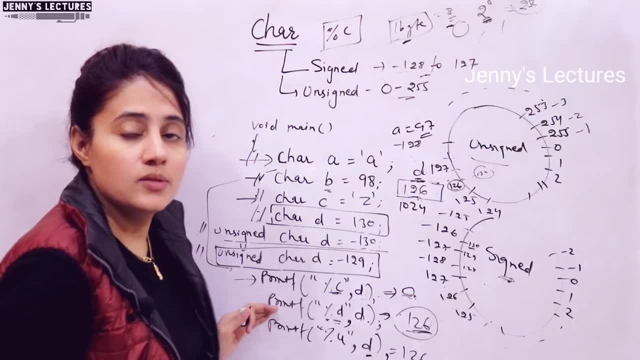 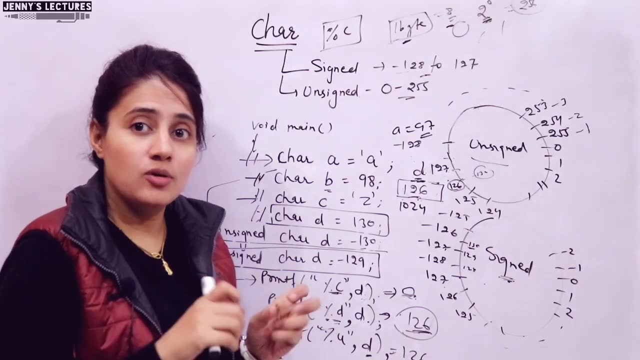 Then go to your system and then check the output. That's a good way to learn programming and to enhance your programming skill, And that's many students ignore this point- Dry running of a program, writing a program with pen and paper, Right. 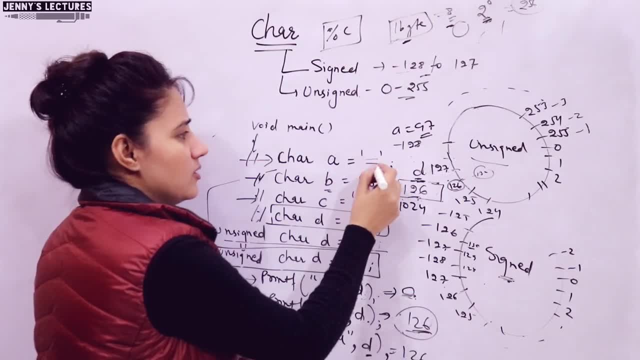 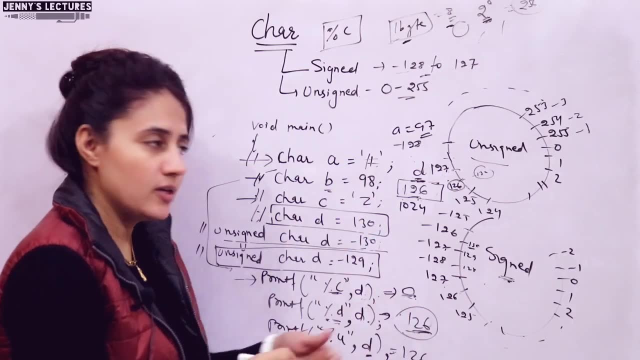 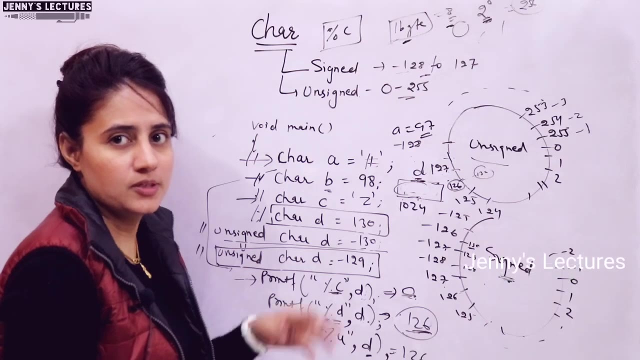 And if you print- suppose, if you suppose here, store any symbol like hash, I'm storing So corresponding to hash- some code is there in a sky. that code would be stored here. When you will print this with percentage C and percentage D, you can check the output. 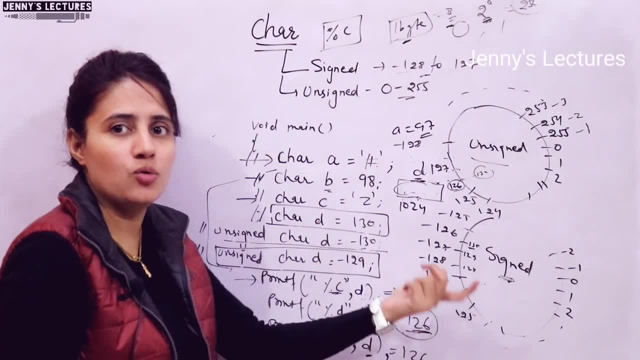 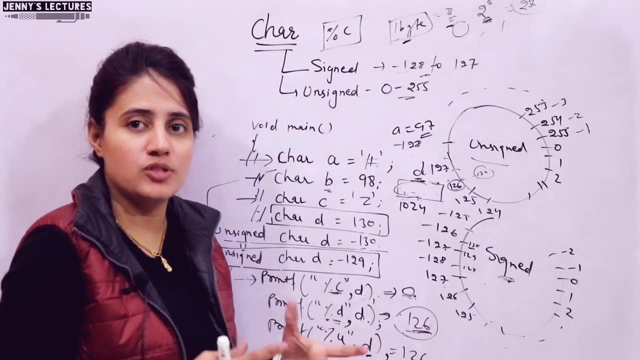 In percentage C, it will print the character. when you will print with percentage D, it will print the corresponding value: decimal value. So now that's exactly how characters and symbols are to be stored in computer memory using those standard codes. So now that's it for this video. 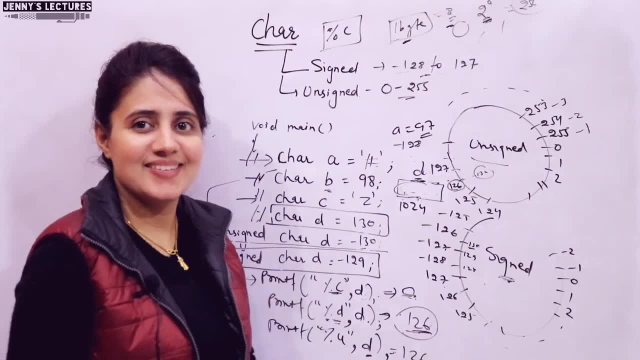 Now I'll see you in the next video. Till then, bye, bye, Take care.